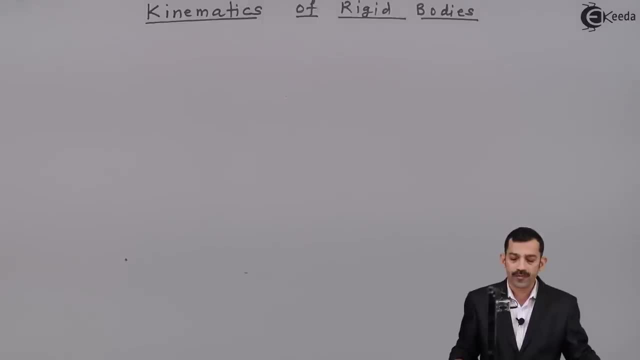 body part. here. rigid body we will say the bodies of any size or shape. when any body rotates, then such a body is considered as rigid body for the analysis of motion. That means, if you take a huge body, maybe you can say a plane or a helicopter, and which? 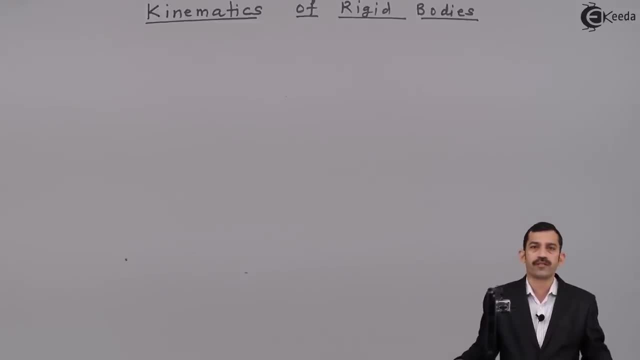 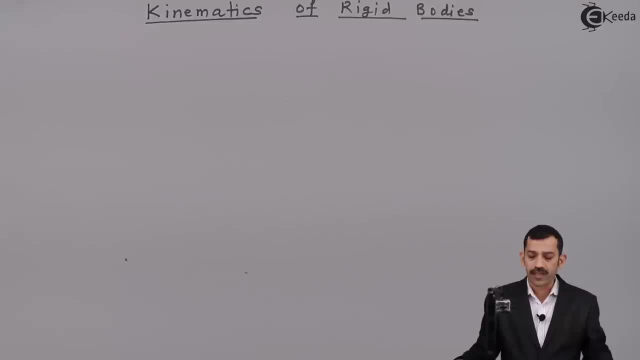 it rotates about some point. That means in this case, in kinematics of rigid bodies. bodies rotate somewhere and without considering masses and without considering forces will analyze its motion. As bodies rotate, some angular terms comes into picture. Angular terms are what? Linear displacement, 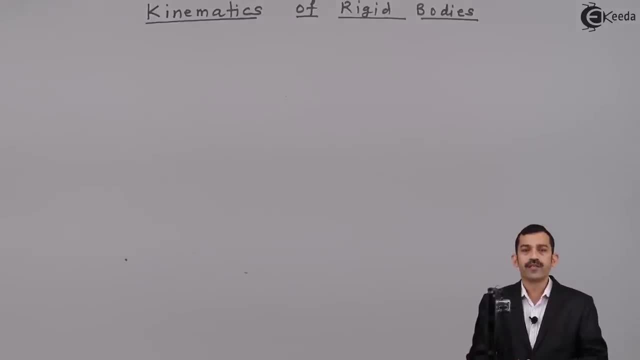 Linear displacement is S, Angular displacement is theta. Linear velocity is V. Angular velocity is what Omega And linear acceleration is A. Angular acceleration is alpha. That means you have to deal with here mainly with angular quantities. Now, if we will assume just here, 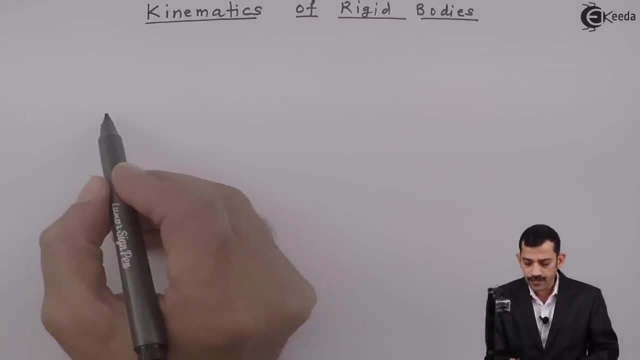 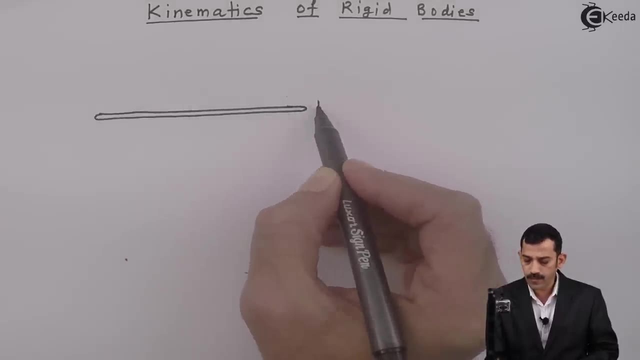 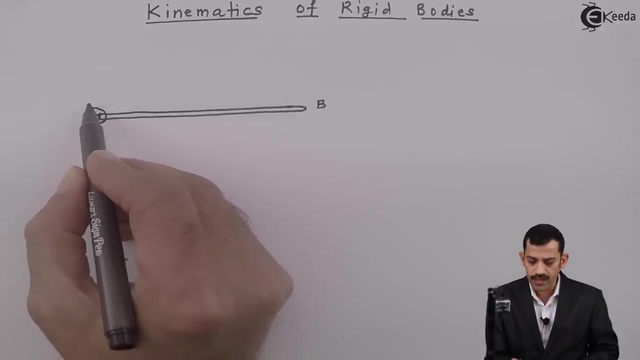 a 1 bar AB. Now this one is a var AB. Which one is hinge supported at A, This one is hinge support. That means at this end, as there is hinge support, rotational motion is allowed If. 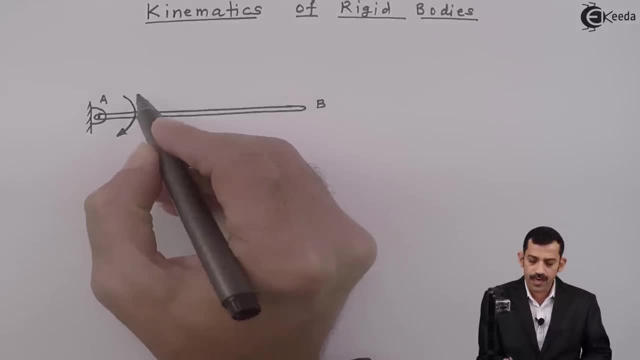 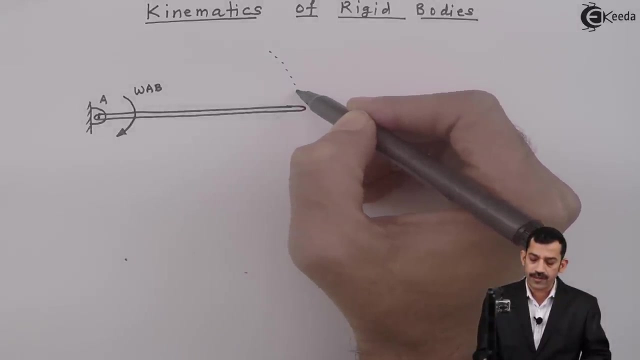 how it is presented like this: one is a direction of angular velocity. What does it represent about point a with some angular velocity, omega ab, if bar rotates about this point, this end b traces a curved path, or you can say arc of a circle right. and for one relation you can say: 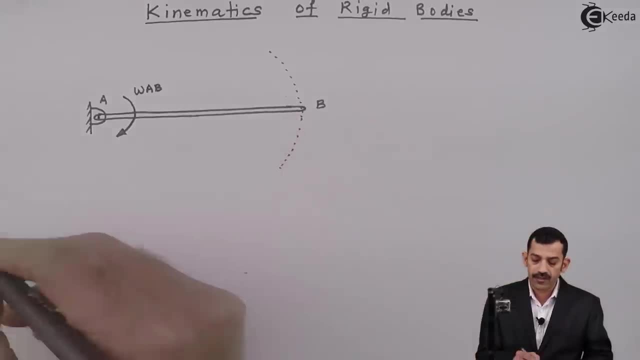 if bar rotates, then end b traces a circle of radius equal to length of bar ab. in curvilinear motion, what we discuss, the linear velocity of any point, is always tangent to the path. that means, as point b lies on this path and this bar rotates in clockwise direction. 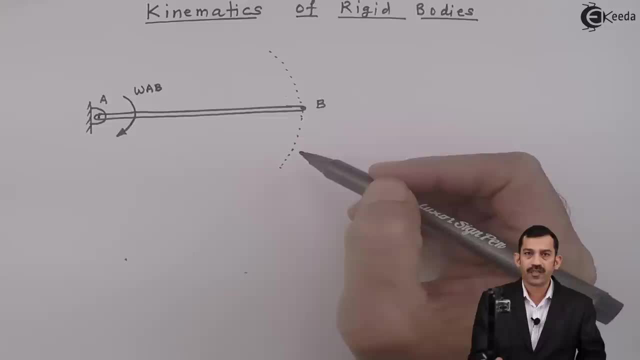 at this point it will represent tangent. tangent means the line which just touches the curve at point b, if you draw, tangent means perpendicular to ab, because at point b, Publisher, If we join it to point A, which is here center of circle, here, or center of this arc, AB represents normal. 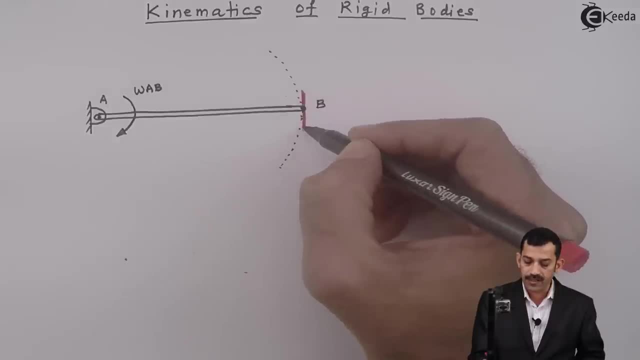 Let me see here: if I draw a line, tangent means perpendicular to this AB, what will get here? vertical line: This line is always tangent to the path, Or you can say it is perpendicular to bar AB. Similarly, linear velocity of any point on a rigid body is perpendicular to radius of rotation. 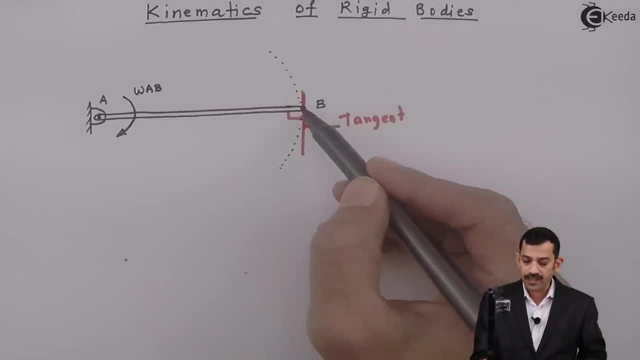 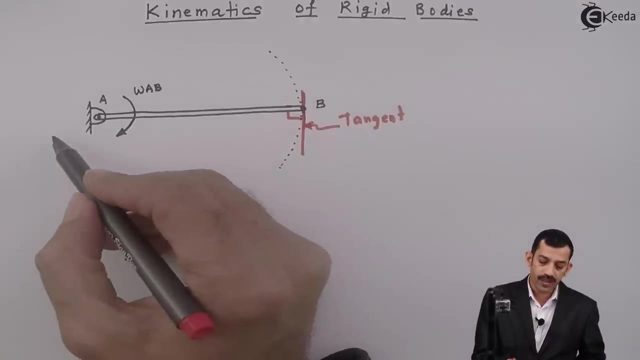 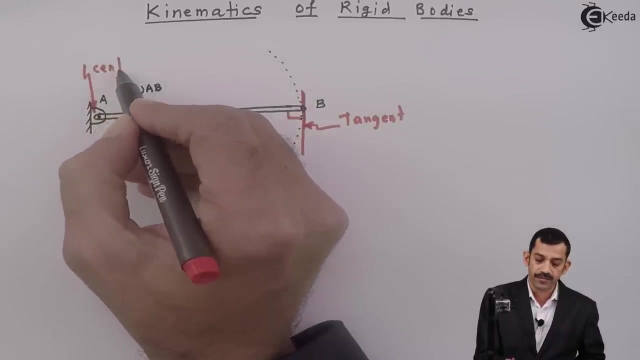 Here radius of rotation means what You are finding, say linear velocity of point B, Now bar, rotates about point A. So this point A is called as center of rotation. This point is center, Center of rotation. Point A is center of rotation. 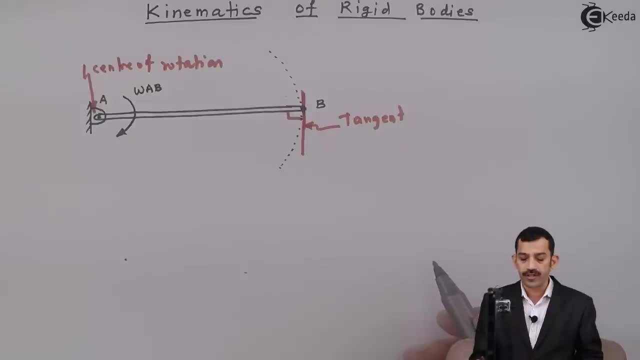 If you want to find out linear velocity of any point on rigid body, say AB, this point B. if we join to point A, this length AB is called as radius of rotation. That means for point B, radius of rotation is length AB. 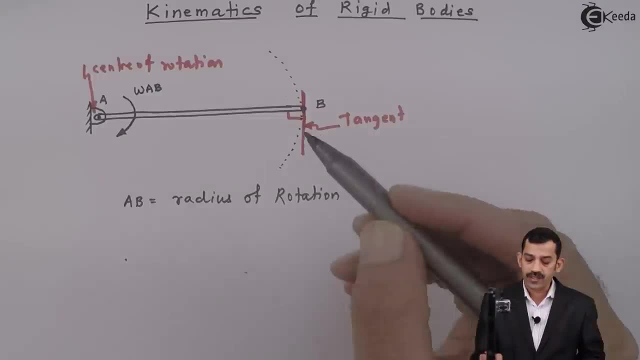 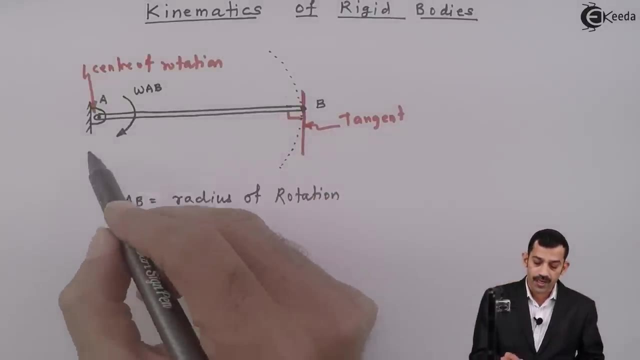 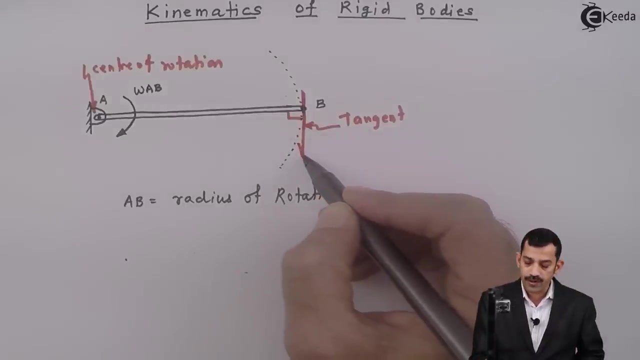 Linear velocity of any point on a rigid body is perpendicular to radius of rotation to this angle is 90. That means this is along tangent. Omega is clockwise. That means B and B has to move in downward direction. Therefore, linear velocity of point B is in vertically downward direction. 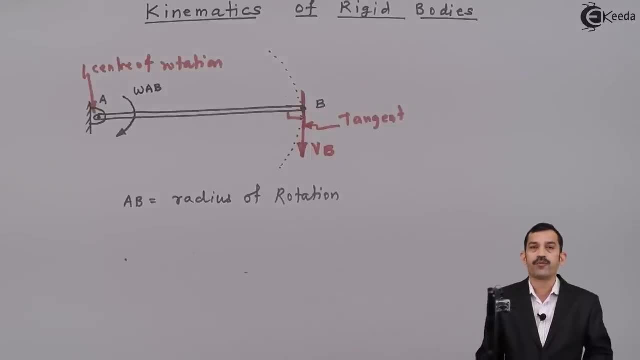 This one is VB. That means linear. velocity of any point on a rigid body is perpendicular to radius of rotation And in the same sense of omega. always. Now, during motion, what will be the position of rod AB will take now, initially horizontal? 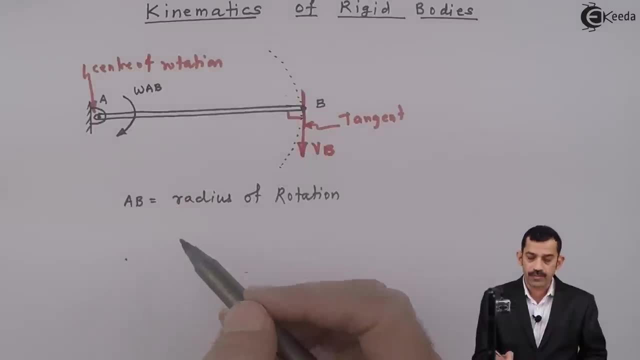 After some time. say, rod is inclined at 30. Next again bar is inclined at 60 degree. Then it becomes vertical. Position of center of rotation does not change When during motion. position of center of rotation does not change. 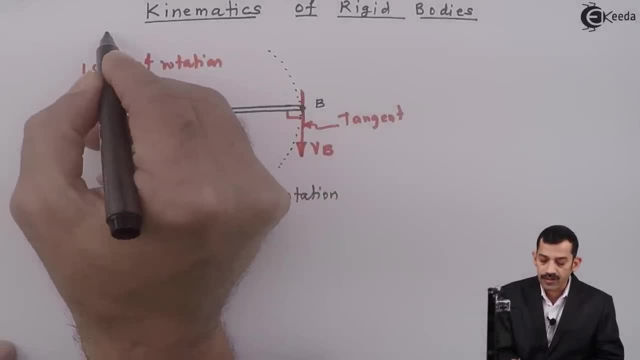 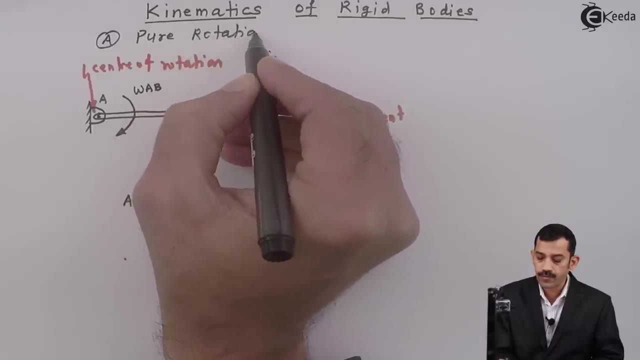 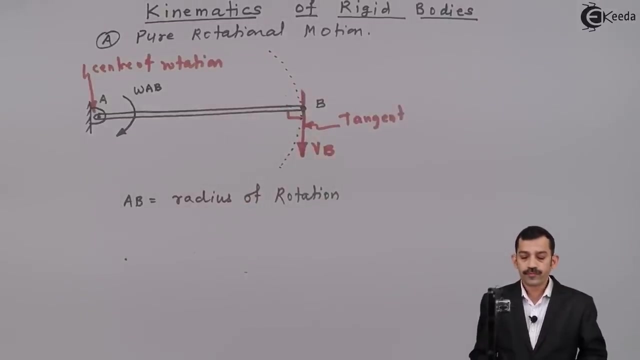 then such type of motion is called as what Say VB, Type A, It is called as pure rotational motion. Which type of motion is called as pure rotational motion? During motion, a position of center of rotation remains fixed, which does not change. 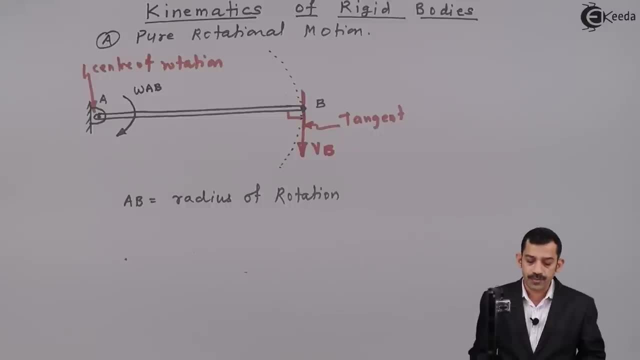 Such type of motion is called as pure rotational motion. In pure rotational motion now, bar rotates about point A. A is called as center of rotation, And distance of any point on a rigid body from center of rotation is radius of rotation. 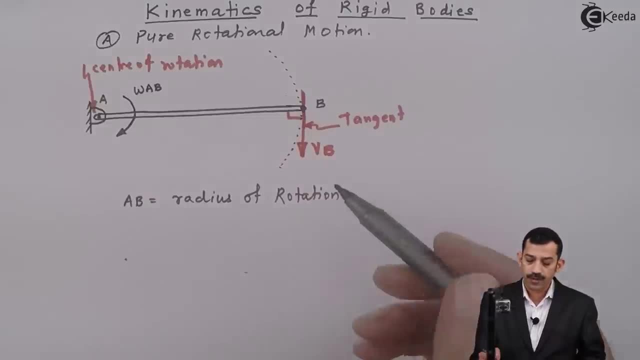 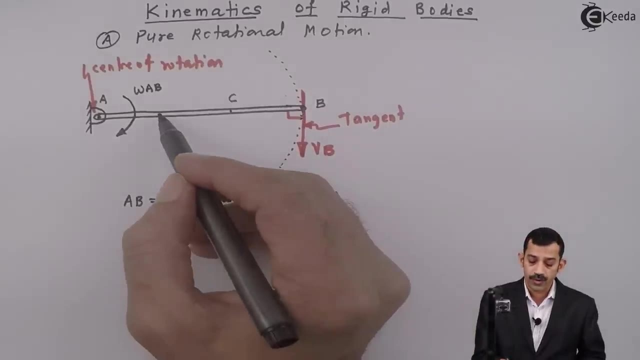 For point B, radius of rotation is AB. If I locate some one more point here, say point C, AC becomes radius of rotation for point C. If I locate here point AD, AD represents radius of rotation for point D. Linear velocity of any point on a rigid body is perpendicular to radius of rotation. 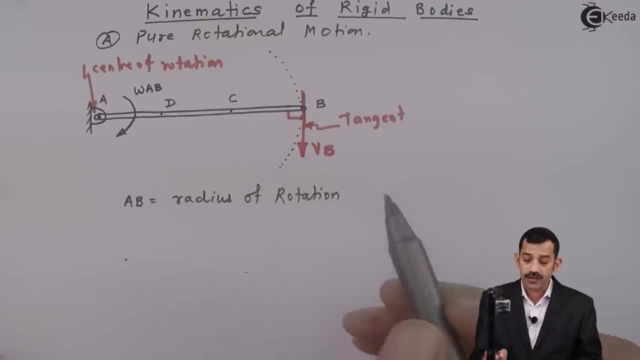 That means VB is what Downward For point C. if you want to find out, linear velocity of point C is perpendicular to radius of rotation. That means here what will get? Perpendicular to AC, In the same sense of omega, what will get here? 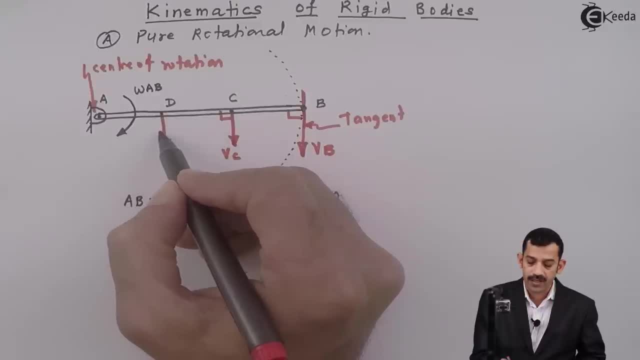 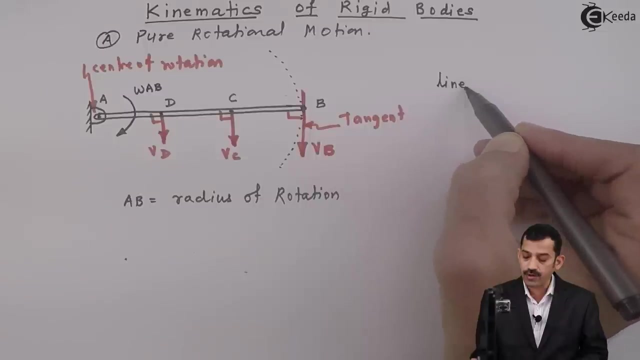 VC, Radius for point D becomes AD, Linear velocity perpendicular to radius of rotation. What will get here? VD? So you will get what? Linear velocities of such points? linear velocity of any point- this is very important. linear velocity of any point on. 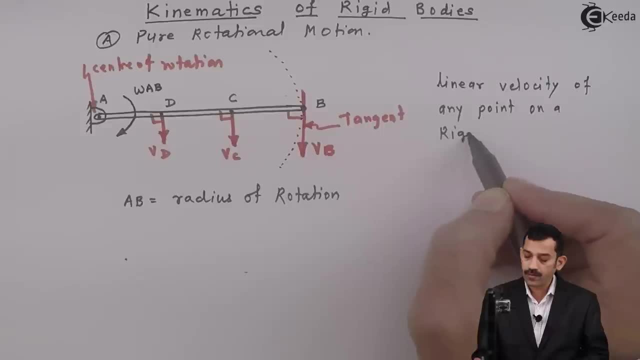 a rigid body is always perpendicular to the radius of rotation and, in the same sense of the, the angular velocity. when you will solve any problem and if you want to represent linear velocity of any point, what is most important, linear velocity of any point on a rigid body is perpendicular to radius of. 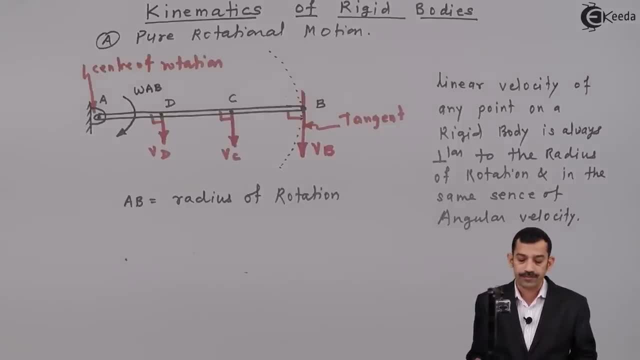 rotation and, in the same sense of angular velocity, omega, clockwise linear velocity is. if same bar, I will do can added what to fully the linear velocity of any point in the same 上 we explore? is it realize what is what? v equal to r, omega, in this case, radius of rotation is what? for point b, radius of rotation. 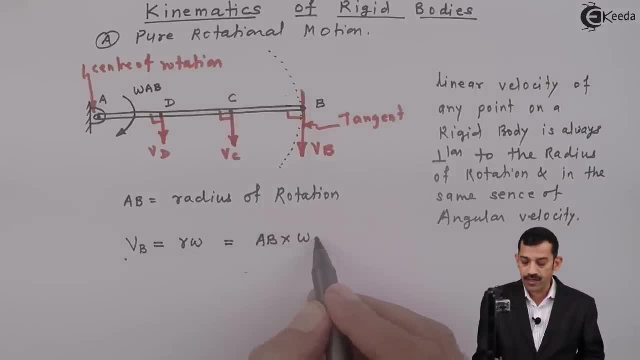 is what ab, omega is of bar ab. that means vb equal to ab into omega ab. similarly, linear velocity of point c, if you will find out what is the radius of rotation that is, ac. therefore here, ac into omega ab. linear velocity of point d, if you want to write again radius of rotation, distance of 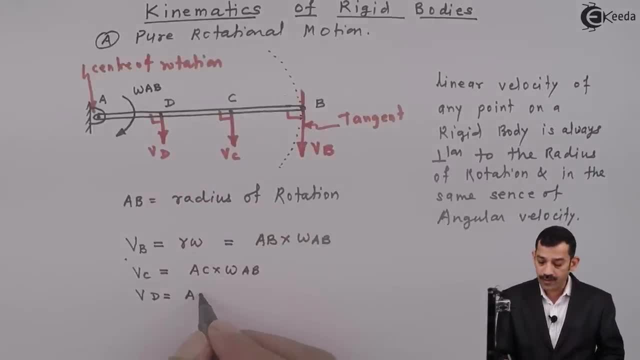 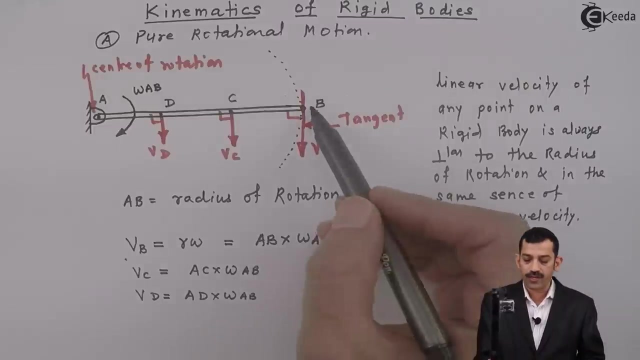 which point, point d from center of rotation. that means what ad into omega ab from this one. if you just analyze out of vb, vc and vd which velocity is maximum. so vb is maximum. linear velocity of point b is maximum. you, because radius of rotation for point b is maximum. for other points radius of rotation is less. 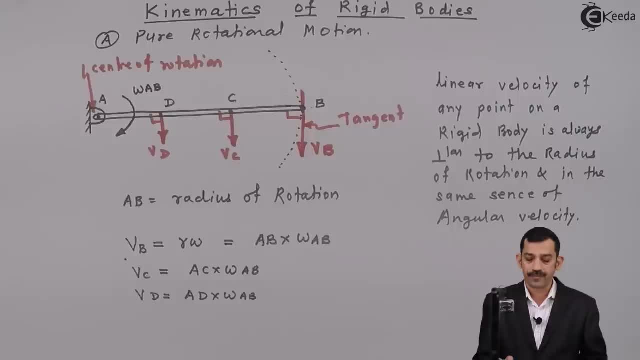 that means vb is maximum. next is what vc? again, vd is less than vc because radius of rotation reduces. that means, as we will move towards you can say, center of rotation, linear velocity of point decreases because radius of rotation decreases. people find out then what is linear velocity of. 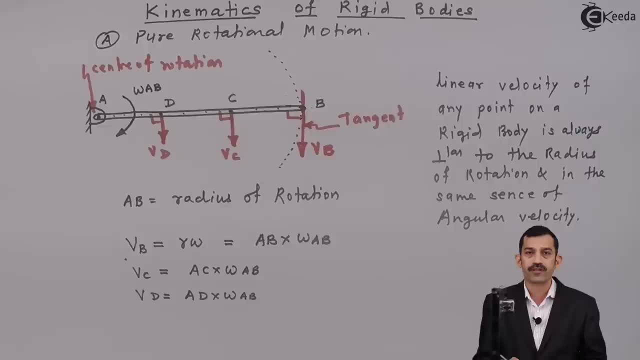 point a, the answer must be zero, because the radius of rotation is what zero? or you can say the point: such a point on a rigid body whose linear velocity is zero is called as center of rotation or characteristics of center of rotation. is what point of zero linear velocity is a center of? 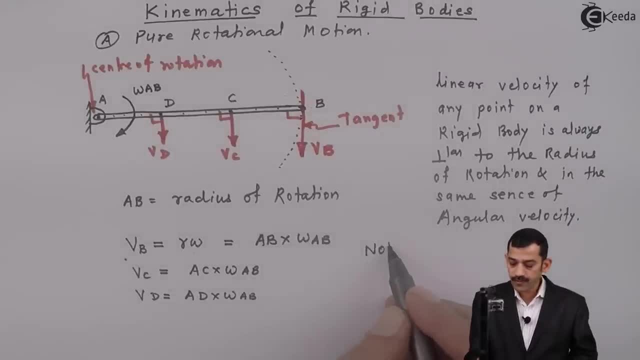 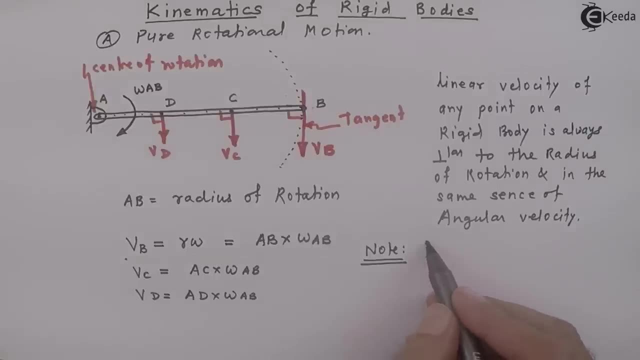 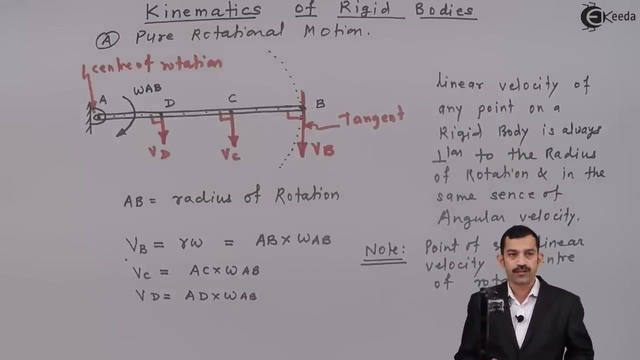 rotation. let me- this one is very important, actually in any problem, if you want to identify which one is the center of rotation- the point of zero linear velocity, point of zero linear velocity is center of rotation, is center of rotation. that means what we discuss is pure rotational motion. in pure rotational motion, center of rotation, its position remains fixed. 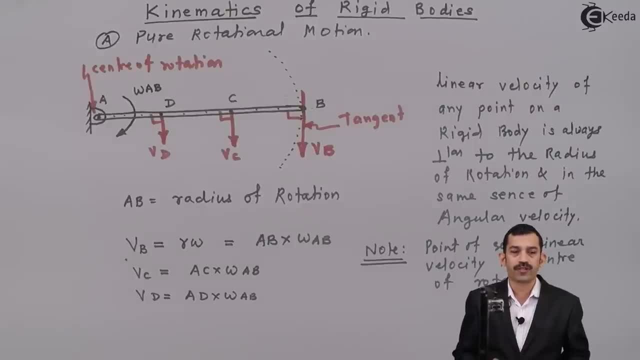 or the motion in which position of center of rotation remains fixed is called as pure rotational motion. linear velocity of any point is always perpendicular to radius of rotation and in the same sense of angular velocity as linear velocity is perpendicular to radius of rotation. can you say radius of rotation is perpendicular to radius of rotation? 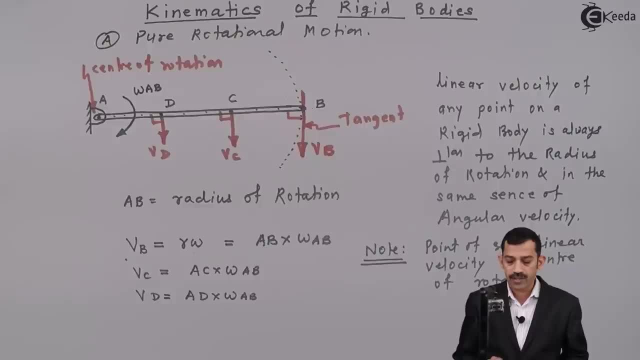 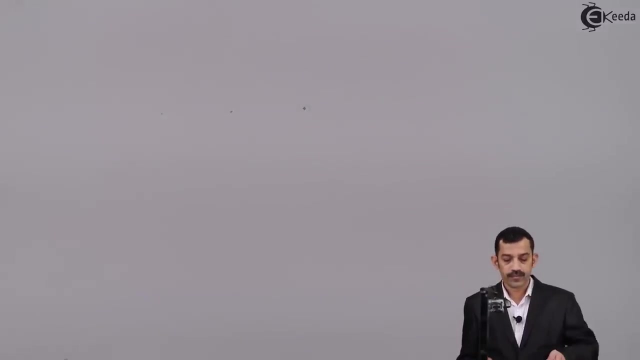 to linear velocity. one and the same thing. because if you know linear velocity of any point and from that one, if you want to represent where is the center of rotation first, will represent what radius of rotation which is perpendicular to linear velocity. so this one is simple type of motion. next motion will see now how, if we will assume, say this one. 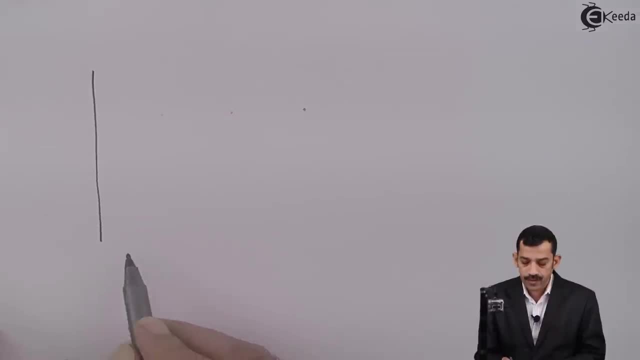 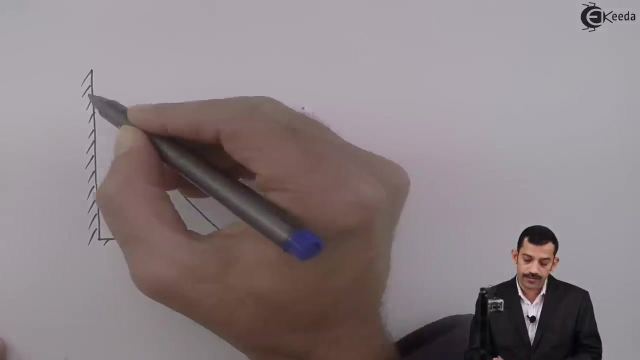 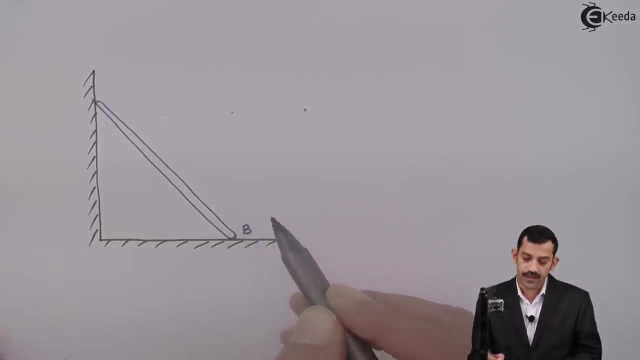 is a vertical wall, then this one is a ground, rigid surface. wall is a rigid surface, ground is a rigid surface. Now, if we will represent, say there is one bar, one end is resting against vertical wall, other end is resting on ground. Say this one is again rod AB. Say this end is B, this end is A. 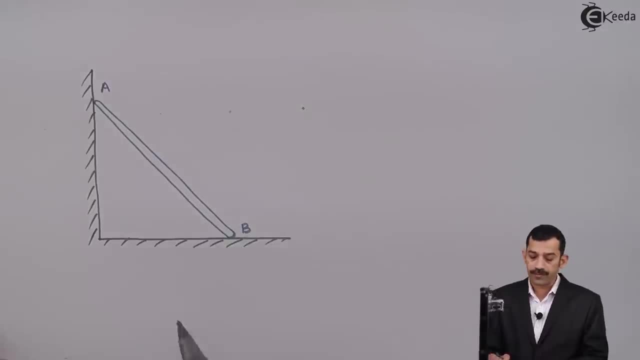 So bar AB Now, assuming frictionless or smooth surfaces and this rod moves with some velocity, Definitely end A will slide in downward direction, end B will slide in rightward direction. That means, if I will represent what is the velocity of point B, what will get here? VB Velocity of point A: you will get in vertically downward direction. 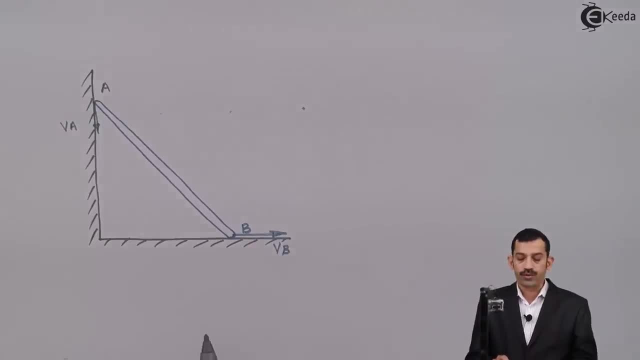 see, this is what va now, as you know, va downward, vb downward. both the points a and b lies on same rigid body, say rod ab. that means both the point lies on same bar ab. now, if you want to represent, where is the center of rotation, the from each velocity? 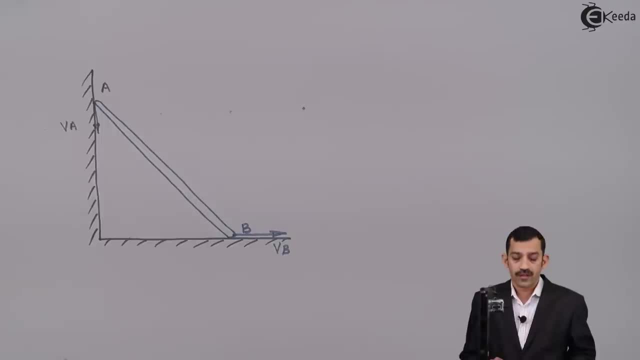 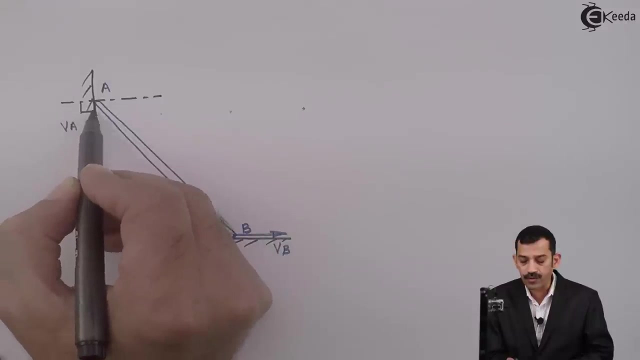 first we will try for radius of rotation. as you know, linear velocity is perpendicular to radius of rotation. can you say radius of rotation is perpendicular to linear velocity? say for point a, you know linear velocity, vertical, that means radius of rotation. if you want to represent, i will draw here a line which one is perpendicular to va. that means on this line, somewhere you must. 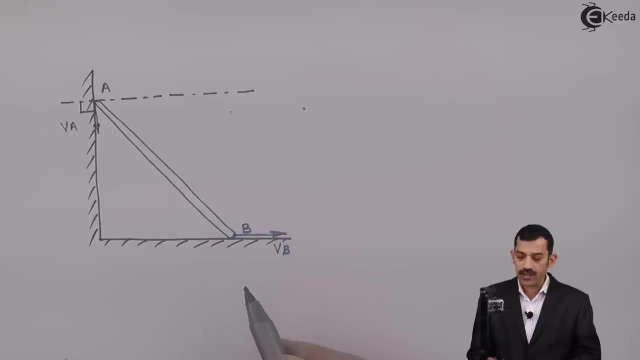 get what center of rotation? similarly, vb is in horizontal direction. if i will represent here perpendicular to vb, this linear velocity, this angle is 90, so on this line you must get center of rotation, because center of rotation always lies on radius of rotation and radius of rotation is perpendicular. 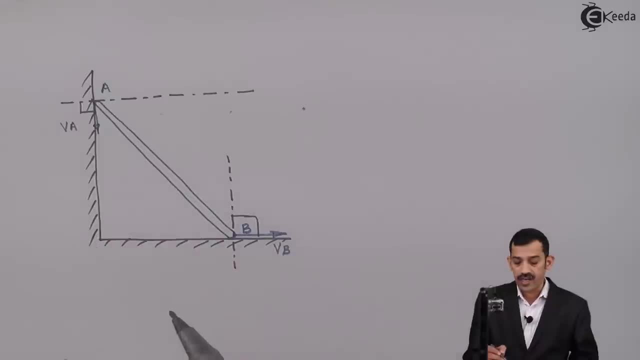 to linear velocity. as you know, va and vb, these are linear velocities of ends a and b of rigid body ab. if you draw perpendicular to va on this line you must get some where centre of rotation line represent radius of rotation. as perpendicular to vb drawn on this line, you must get some center of rotation where both the condition gets satisfy, because 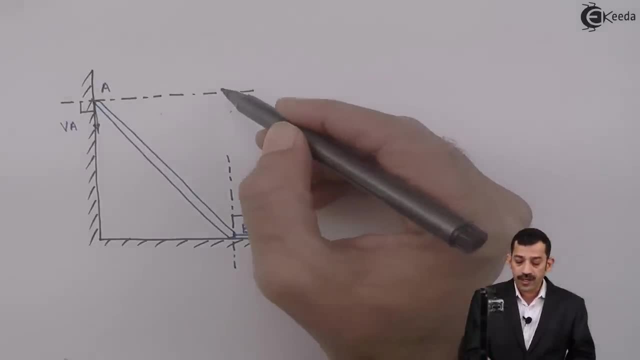 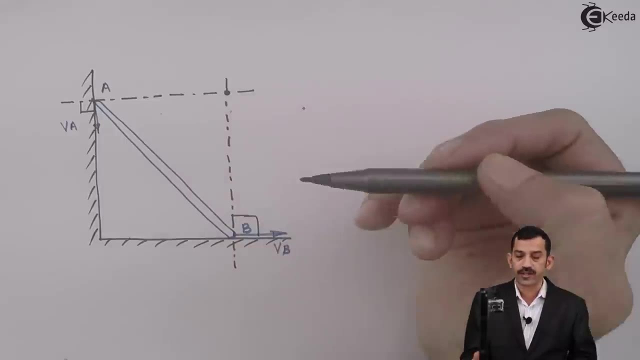 the bar is single bar, that means center of rotation is single, you will get point of intersection of these two bars which satisfy both the condition that means this one is one location where now for va, this line is perpendicular to va. from vb, perpendicular to this line, we will get Congressman. 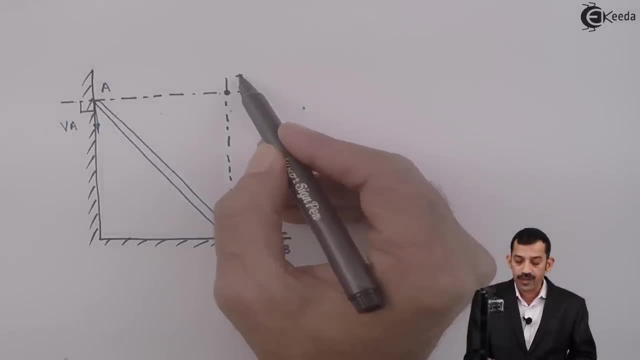 perpendicular to vb. say this one point- i will give some name as point i now point. i is a such a point where both the condition gets satisfied. that means perpendicular to vb and perpendicular to va. i represent, must represent center of rotation, as i represent center of rotation, this point, what we are getting, is called as center of rotation at this position. 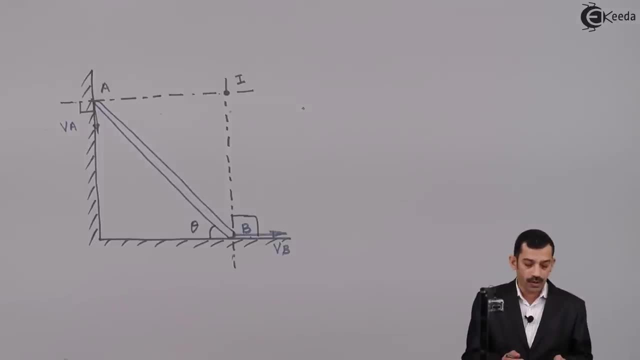 when angle is theta? now at next, one more position, if we will try: a is moving in downward direction or slides in downward direction. b slides in rightward direction. say, after some time you will get position of point b, point a somewhere here. say, name of point is a dash point b moves. 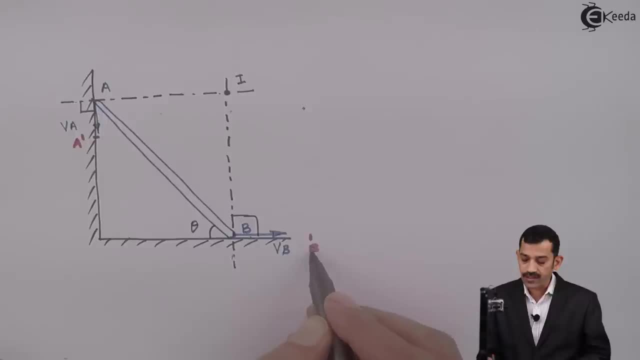 in rightward direction. we will get location of this point as, say, new name will give here b dash. that means: now you position of this bar, ab, is like this: i will join a dash to b dash. motion of body starts from ab now it continues. a moves to a dash, b moves to b dash. that means: 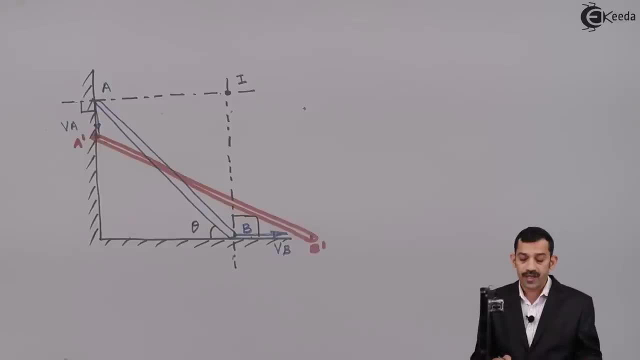 the direction of linear velocity of points equal represent: a continues its motion in downward direction. that means what linear velocity of this point a moves to, b dash, that will get. i will write as a: va dash for this point motion continues. that means vb dash rightward. now if you want to represent center of rotation again, i will draw here what perpendicular, perpendicular. 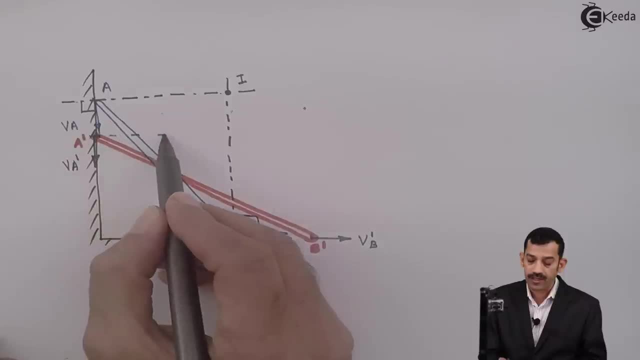 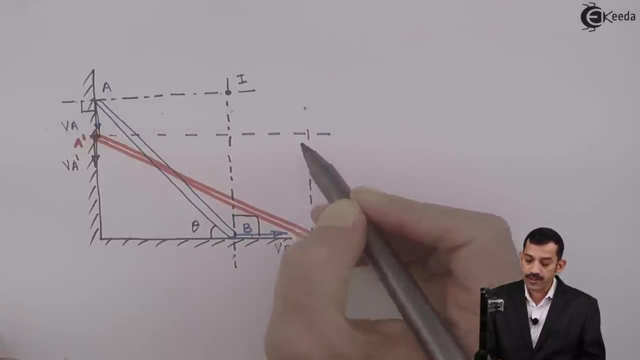 to what va dash. that means what will get here? horizontal line perpendicular to vb dash. if we draw we will get one vertical line. that means now center of rotation is somewhere different. say this point is again i or this point is i2- initial point. what we are getting is say i1. 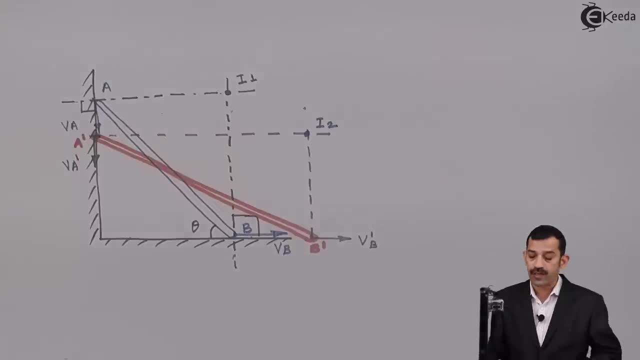 that means this center of rotation point. what we are getting, its position is not fixed at this angle: theta. initially you are getting position as i1 at next angle, which is less than that theta. now you are getting next position, i2. that means at any such position. if we try, you will get. 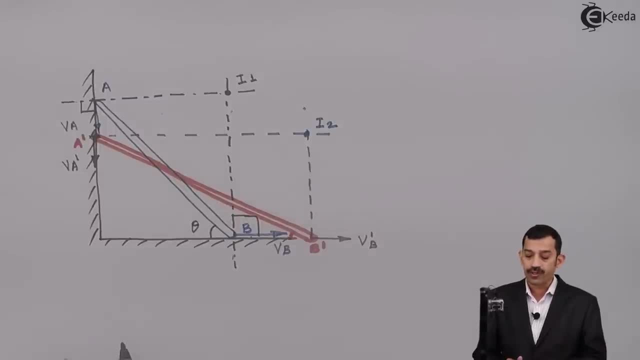 different position of center of rotation. as position of center of rotation doesn't remains fixed, it changes from instant to instant. therefore such a center of rotation is called as instantaneous center of rotation and in short, it is written as icr in figure. while solving problem you want to represent, we will write only by i. 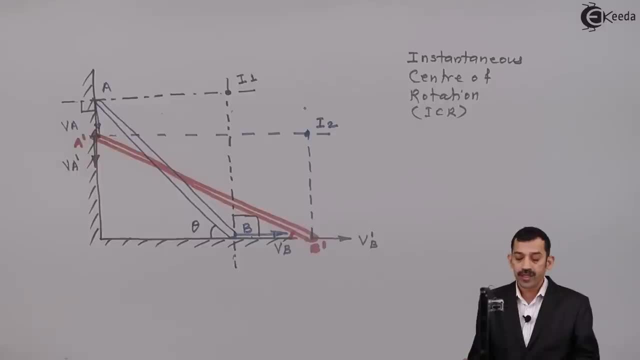 which represent icr: instantaneous center of rotation. that means why this center of rotation is called as instantaneous center of rotation. what point is i1 or i2, these positions you are getting for center of rotation? it is for that particular instant. say at t equal to one. second position is i1. as t increases we will get different position. that means instant. 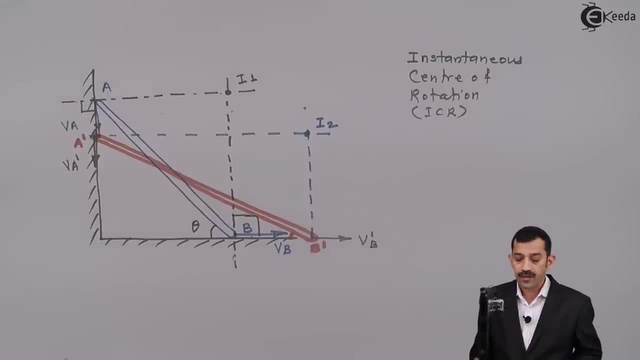 to instant position of center of rotation is different. such a motion, what we are discussing here, which doesn't rotate about some fixed center of rotation, then such motion is basically, it is a combined type of motion and if we will try to represent just here: initial position is ab, say vb is in rightward direction, we will assume end a also moves in rightward. 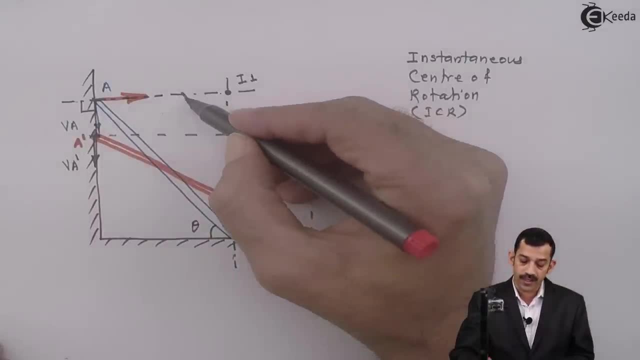 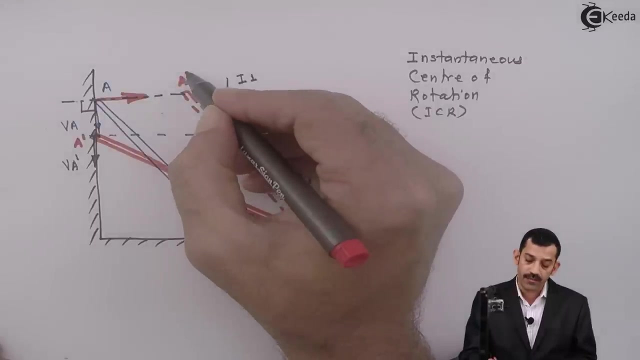 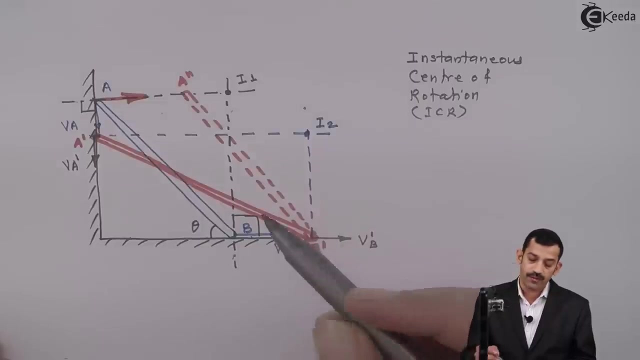 direction, in this direction and what we will get here- say again, intermediate position, something like this. that means which type of motion are considered. here is a translatory motion which moves from a, b to. you can say a double dash, b dash. once you get this translatory motion, imagine at this point, b dash. 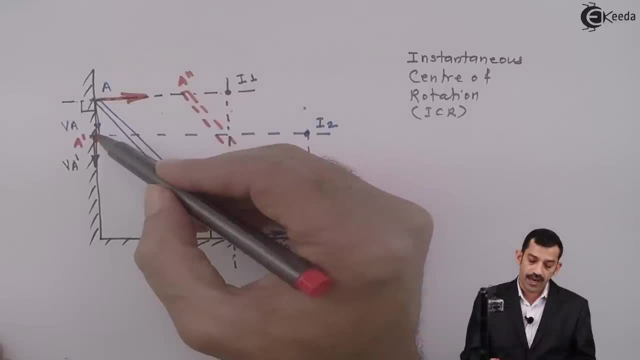 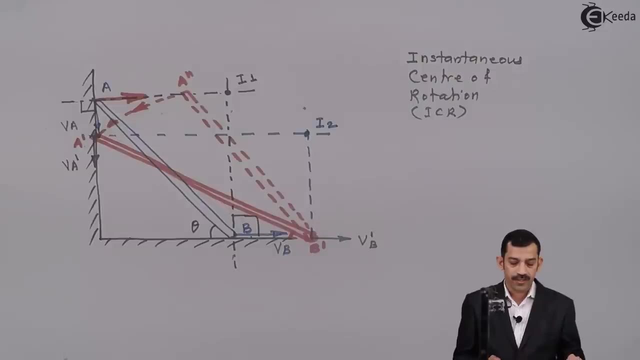 bar, a double dash, b dash rotates and as it rotates, final position. what will get here again a dash from this discussion. can you say what motion we are discussing here is which type of motion? so first there is a translation, then rotation. that means it is a combined motion and a combination. 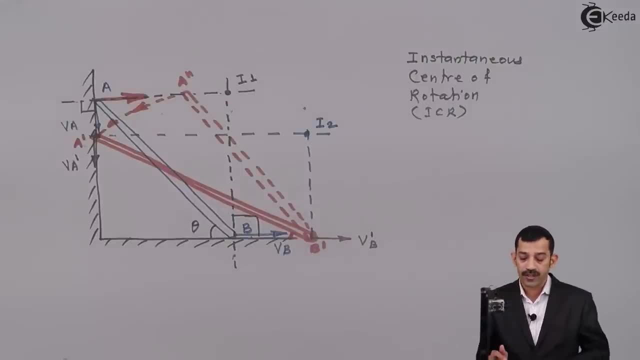 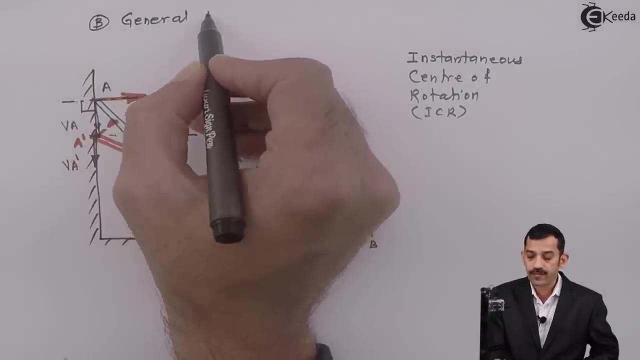 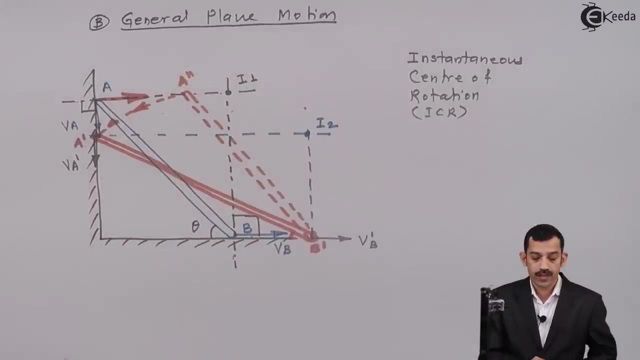 of translation and rotational motion. such type of motion is called as general plane motion. now, general plane motion, this type of motion, it is a combined motion and combination of translatory motion and rotational motion. now, if you want to find out what are the linear velocities of the equation initially, if you take a position as 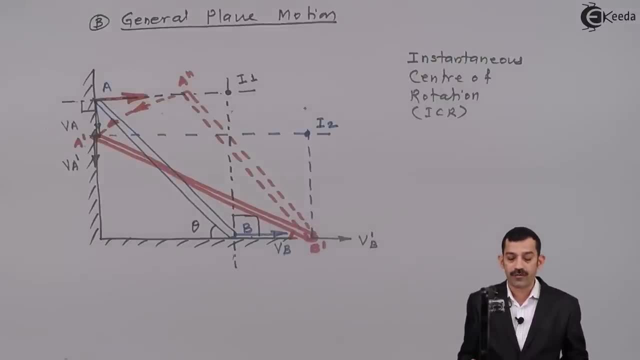 ab for position, ab center rotation is i1. that means at this instant, this motion, 이 egya, you gain. so what you do as i2, you Hipsterب, can be assumed as a pure rotational motion at that particular instant. for example, i1, a, b, what? 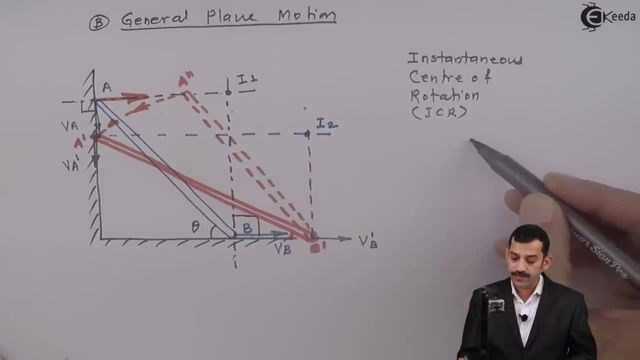 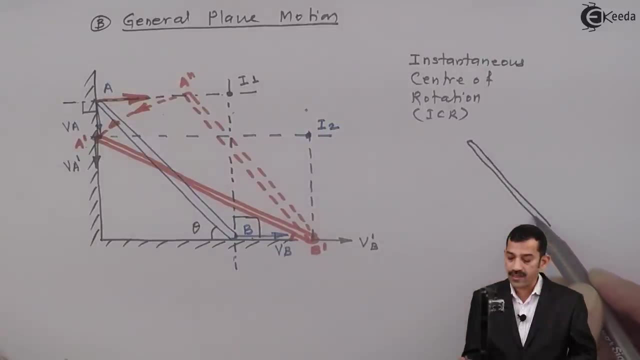 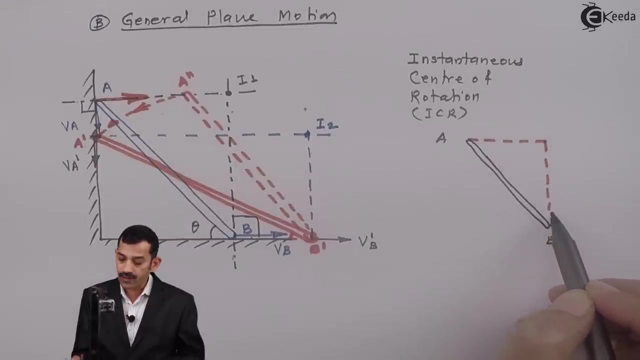 position you are getting, i'll represent here, say this one is what a rod? this end is a and other end is b, and a and b. then you have drawn what perpendiculars- horizontal, this one vertical, and what we have taken is what this point say, this one is hinge. 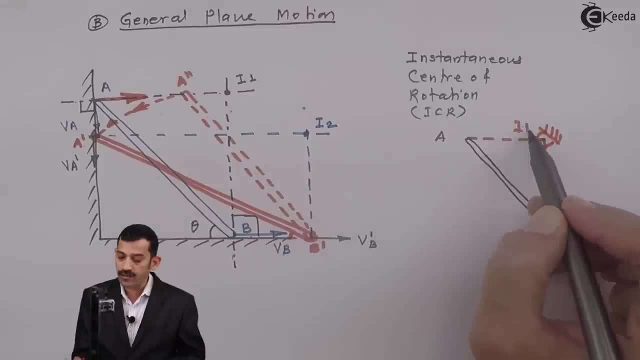 and name of this point is what i1. now you know, v a vertically downward, v b rightward. that means it becomes now easy to imagine. assume it's a triangular plate which rotates about i1. this one is just at right angle and this one is at left angle. so if i want to write from this point, 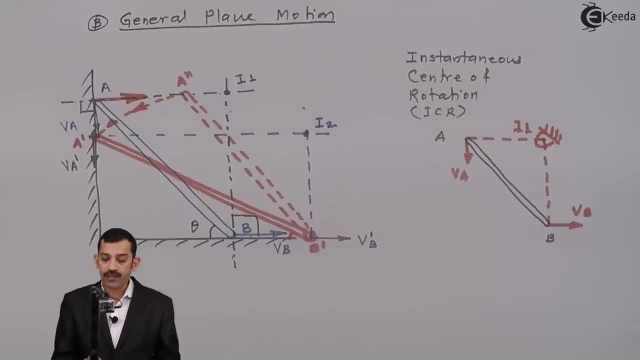 then if i want to write from this point, it must be reach all these points of contact and it must pleding at these points in the form of i1. that is what will be the case if you do needs h min and that instant. you can imagine it like. this can be assumed. this general plane motion can be assumed: 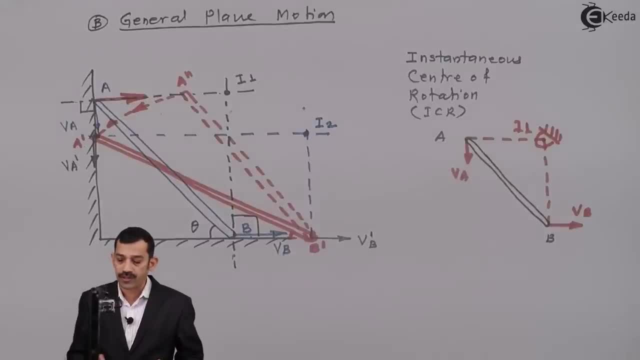 as a pure rotational motion at that particular time instant which is not pure rotational motion at that instant, if you assume you know this one is a pure rotational motion where center of rotation is this hinge i1. now you know va and vb, you may imagine this one is what a triangular plate and 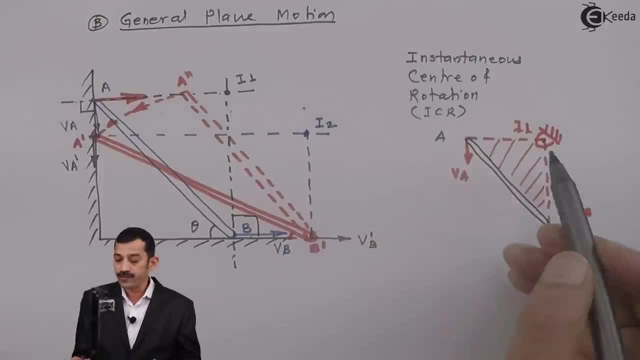 now from direction of va and vb. can you see this bar ab rotates in which direction? anti-clockwise direction, like this omega ab. therefore, now for this case. if we try to write equation, what equation of va will get? radius of rotation into omega? radius of rotation is i1a into omega ab, vb. what? 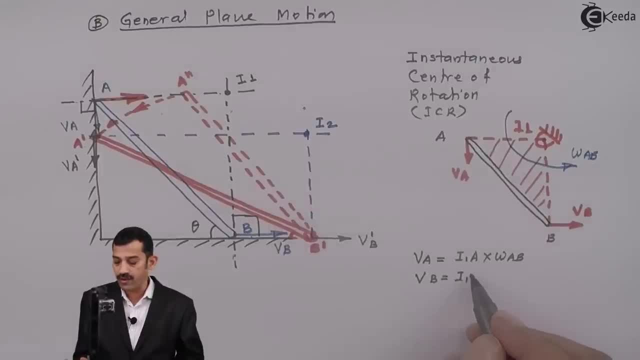 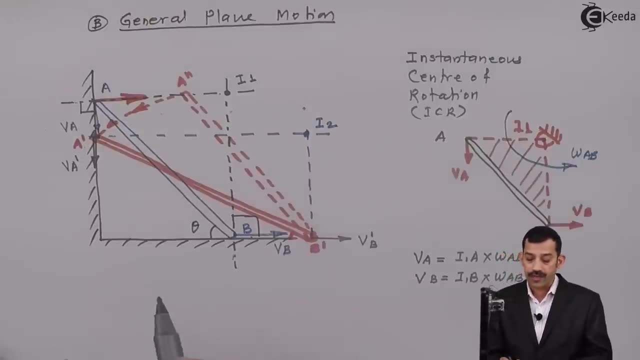 will get here. it's a distance from center of rotation i1b into omega ab. for next position i2. if you want to write what is va dash to va dash is what it's: a distance from center of rotation. that means i2a dash into same bar ab to omega ab. vb dash is what i2b dash into omega ab from this. 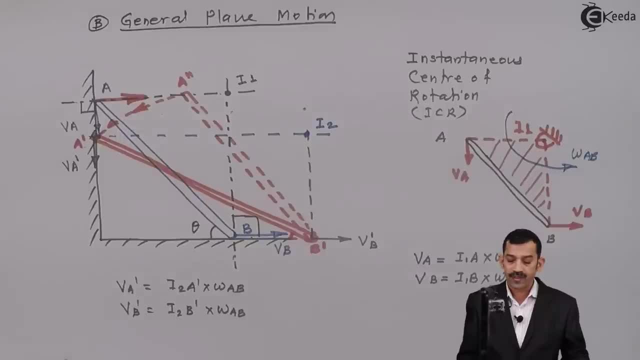 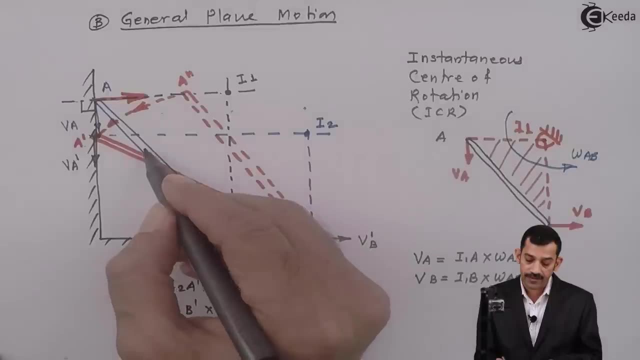 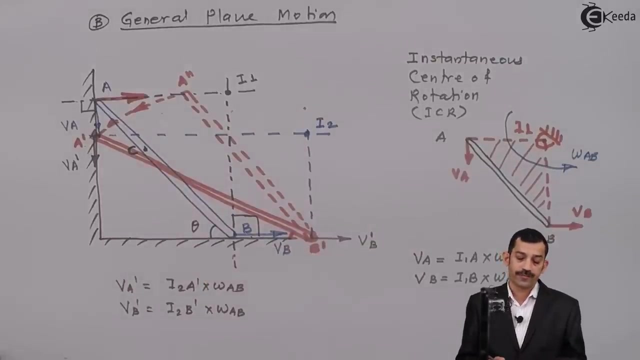 one will get linear velocity of any other point on a rigid body. say on bar ab there is one point c. if you locate here, say this point is what here c on the bar, determine what is the linear velocity of this point c? linear velocity of any point is always perpendicular to radius of rotation. 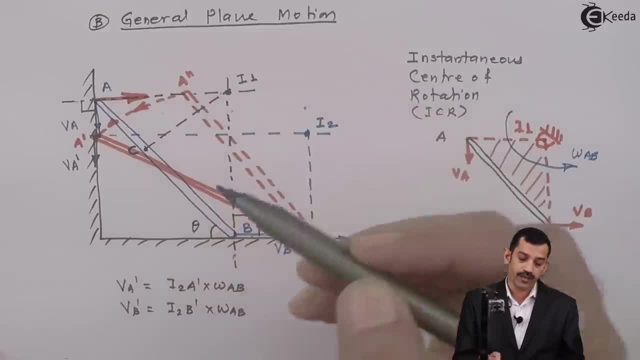 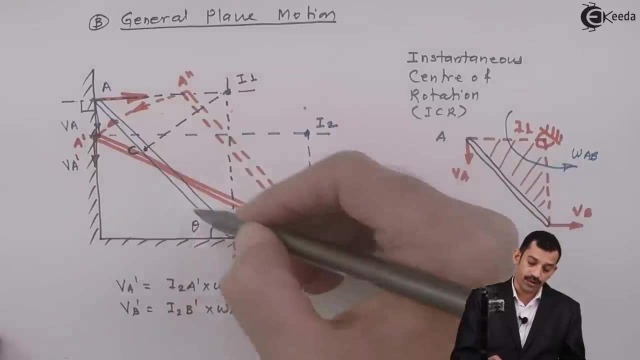 therefore, first i will represent what will join it to center of rotation, and then will draw perpendicular to radius of rotation, and then will draw perpendicular to radius of rotation, perpendicular, perfect perpendicular to i1c. it's not along ab. i'll draw a line, which one is. 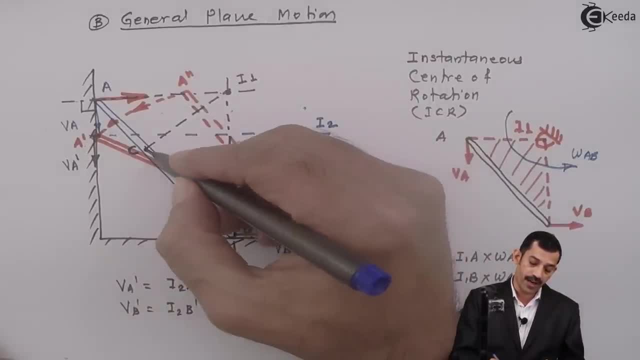 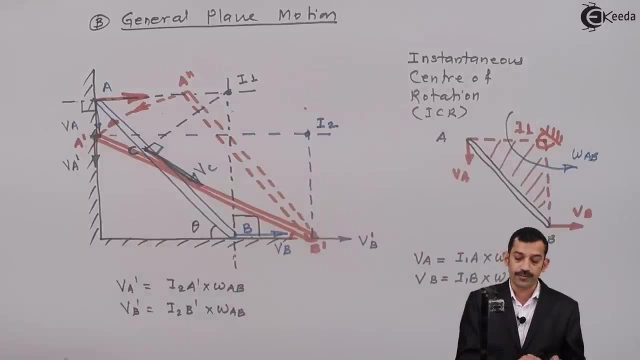 perpendicular, perpendicular toward i1c. say this one is a line, perpendicular right, this one is vc. which is what perpendicular to i1c? that depends on what length each and everything is given from that one linear velocity. if you want to find out. it is perpendicular to this. i1c means radius of. 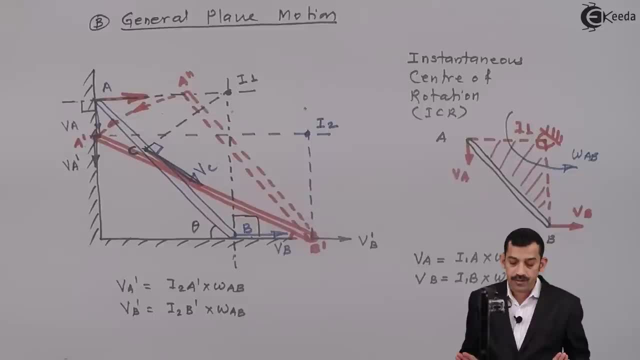 rotation. now, from this one can you conclude like this, if in any you can say rigid body problem, if you know directions of linear velocities of any two points, will draw perpendiculars to the velocity vectors, as we have drawn here: perpendicular to va, horizontal, perpendicular to vb, vertical, point of intersection of these two. 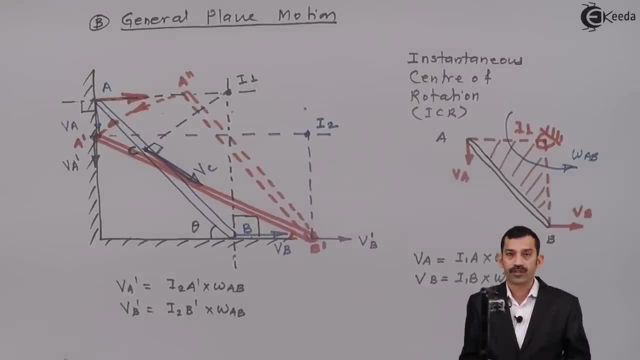 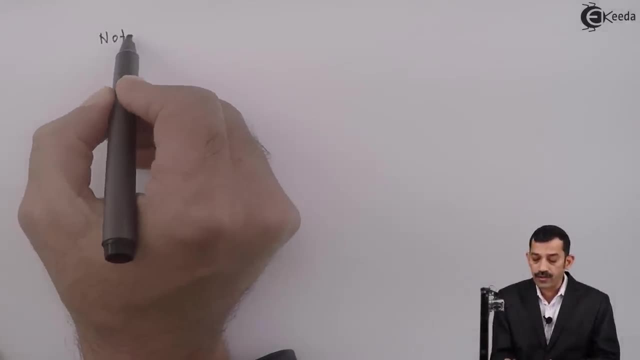 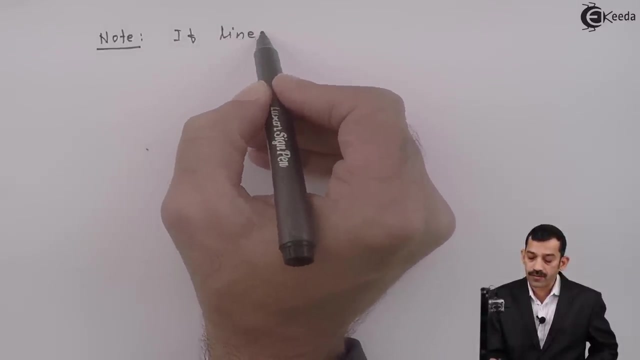 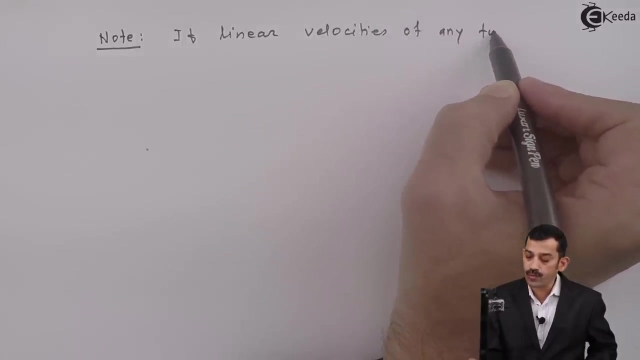 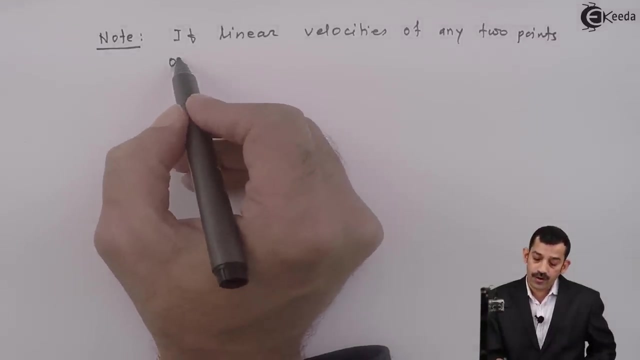 prostrations will draw perpendicular to the velocity vectors as we have drawn here. perpendicular is what you have drawn- represents position of center of rotation. that means- we will write this as a note- if linear velocities of any two points, if linear velocities of any two points on a rigid body. 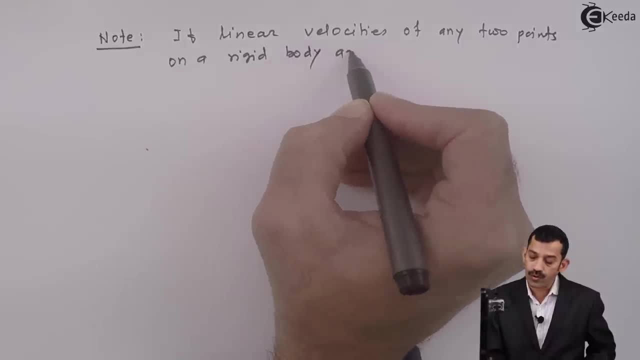 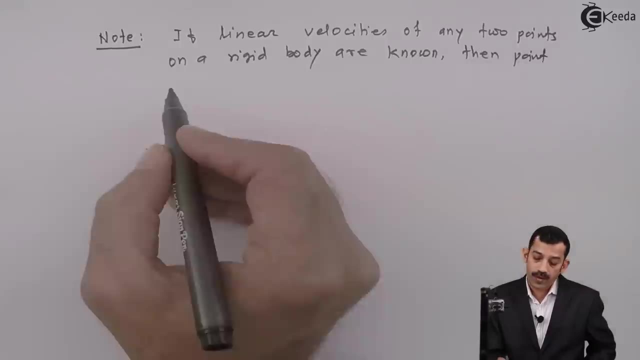 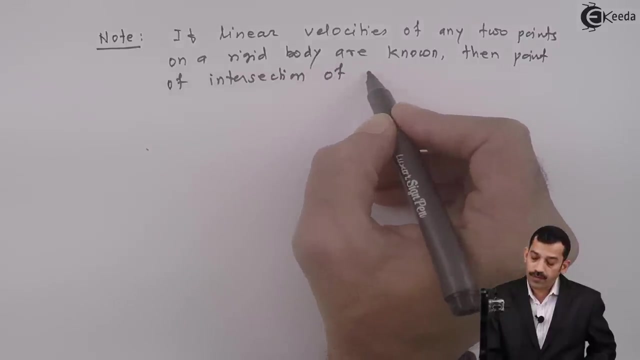 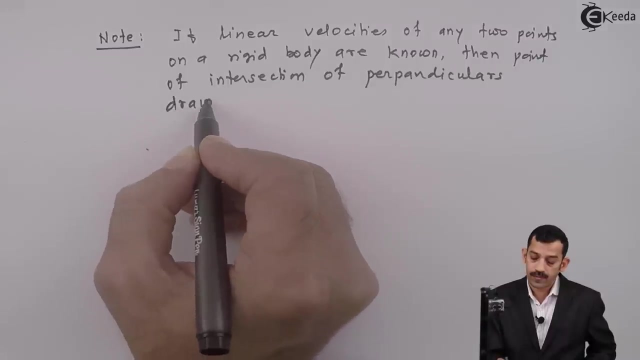 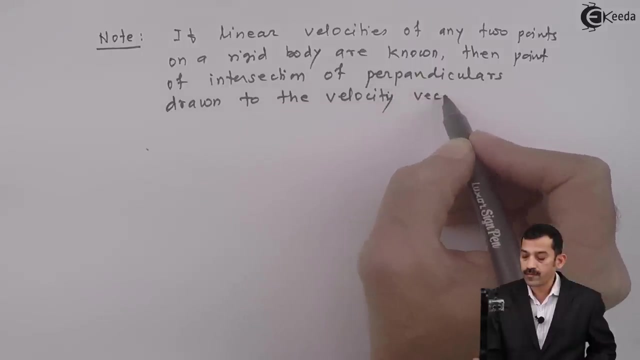 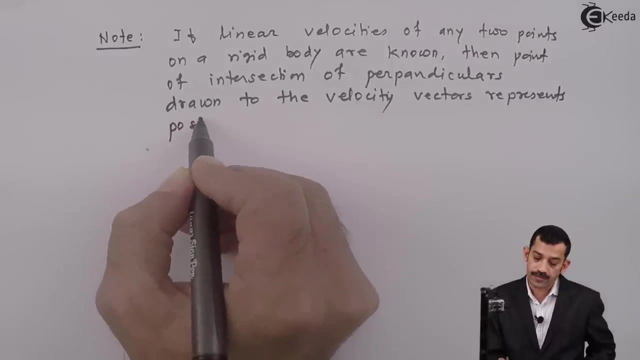 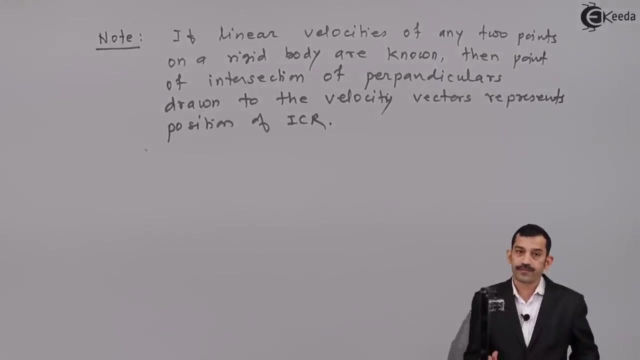 are known, then point of intersection of perpendiculars drawn will be to the velocity vectors represents position of ICR. if linear velocities of any two points on a rigid body are known, then point of intersection of perpendiculars drawn to the velocity vectors represents position of ICR. 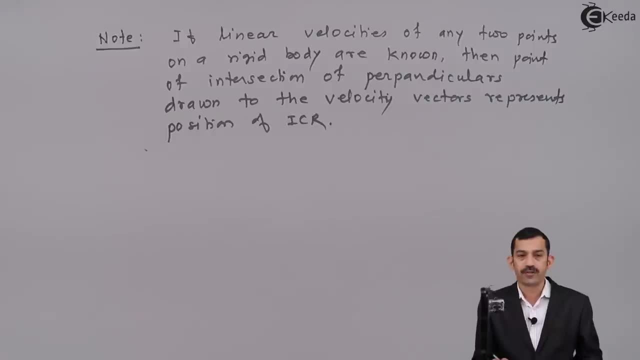 you will get number of such problem. where may be linear velocity of any two points are known. how will locate ICR then? simply, we will draw perpendiculars to velocity vectors. you will get some point of intersection. point of intersection represent center of rotation. similarly, one more type of motion is possible. 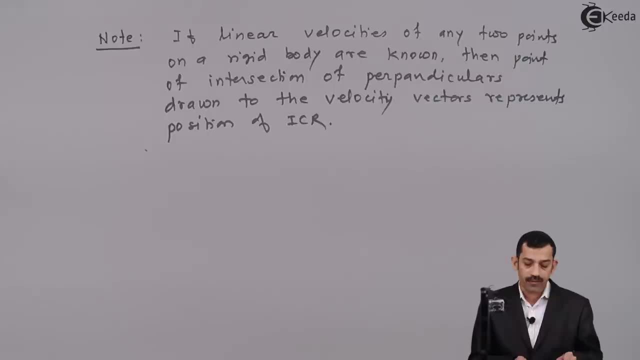 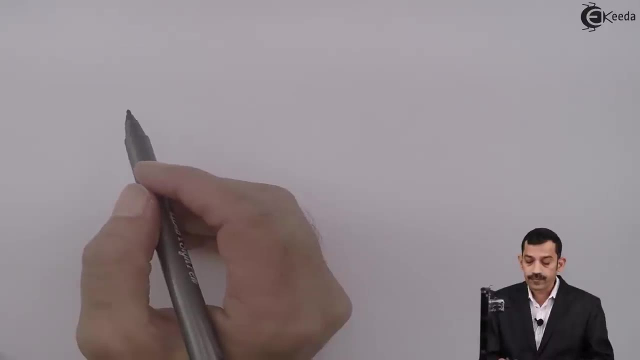 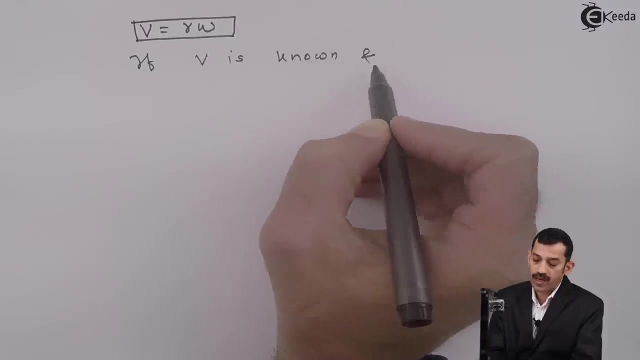 this one is general plane motion. in general plane motion, sometimes we will face difficulties. how to locate ICR? let us see equation v equal to r into omega. this relation is between: in between what linear velocity, radius of rotation and angular velocity, if v is known and omega is known? 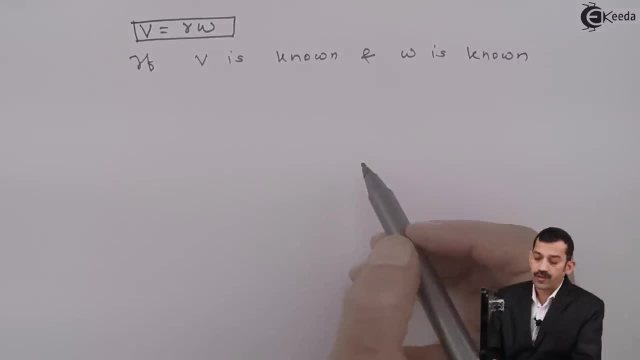 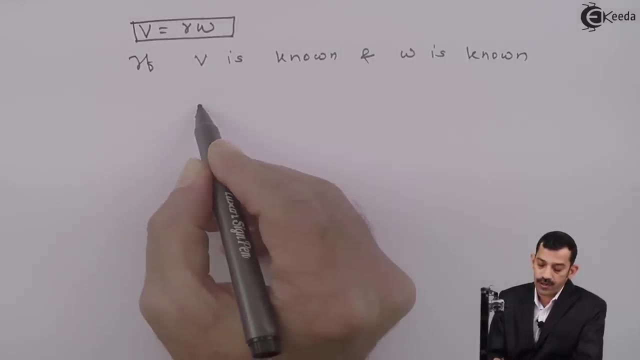 and omega is known and omega is known. if v is known and omega is known and omega is known, then radius of rotation is possible. for example, see this: one is nothing. but what suppose one rod a, b will take say vertical at a and b? hinge is not given. that means motion is not. 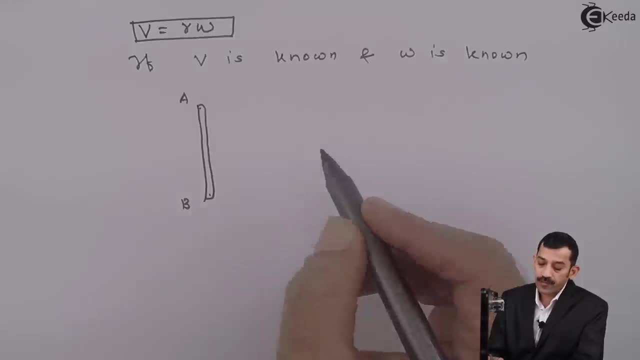 pure rotational motion may be. it is given, velocity is known and omega is known. first we have to decide omega is in which direction, and v is known, so its direction must be known in magnitude and direction. if you know where is linear velocity of point b may be given. 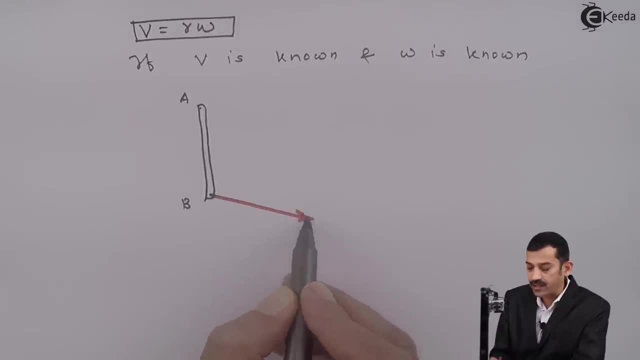 like this: b slides in this direction, v b now as omega is known. you know, radius of rotation is always perpendicular to linear velocity. i will draw here a line which is perpendicular to vb. this line is perpendicular to vb and if it is given omega, that is nothing but in say. 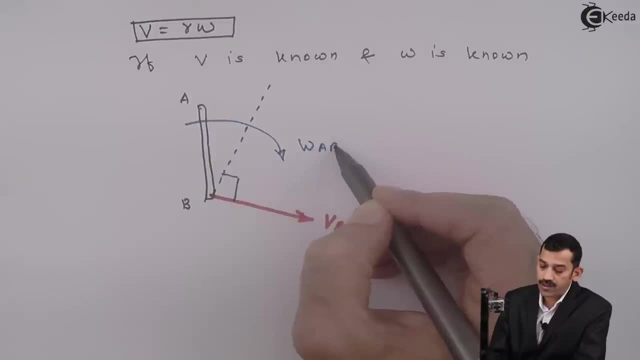 clockwise direction like this. so this one is omega of this a, b. now if you want to find out r, can you say? r equal to what? v upon omega? simply substitute value of v, substitute value of omega. we will get what radius of rotation that means. here you can say: we will locate. 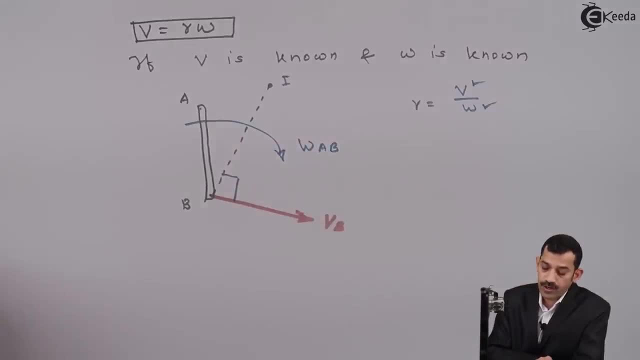 that point as icr. now, if you want to represent what linear velocity of point b may be given as point a, if you want to find out, we will join that point, point i, to point a and if we draw perpendicular to ia, we will get linear velocity of point a out of three term we need. 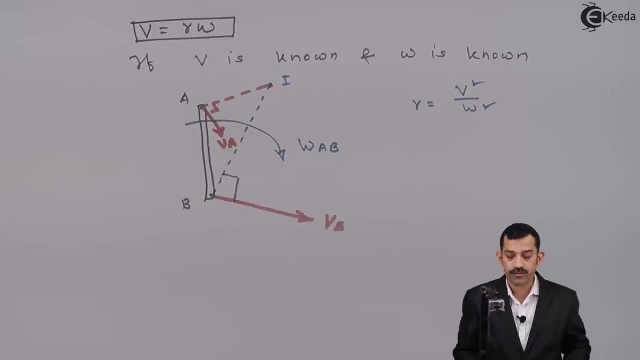 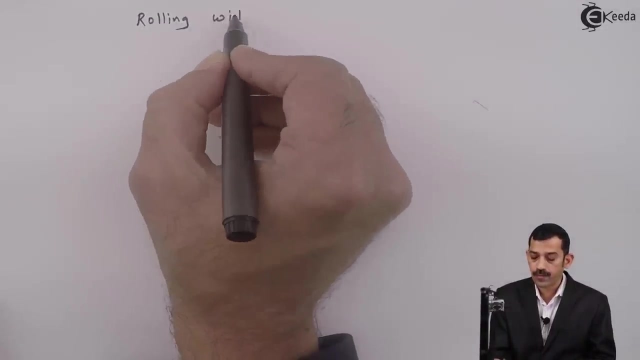 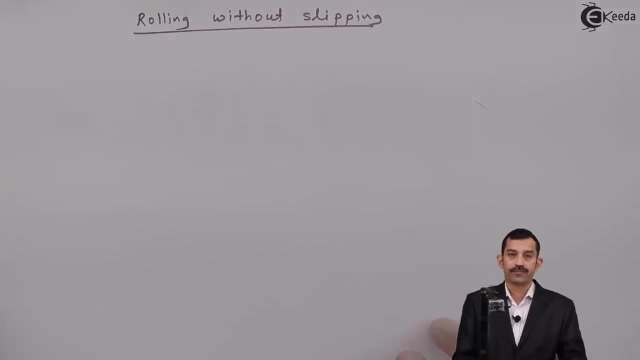 two terms are known easily. we will get position of center, of rotation. next, again important type of motion is rolling without slipping. any circular body may be. you can say wheel of a vehicle. when normally vehicle moves, its motion is always rolling without slipping in. rolling without slipping, say this one is. 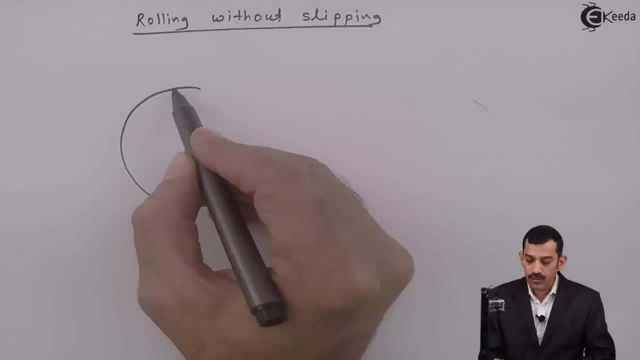 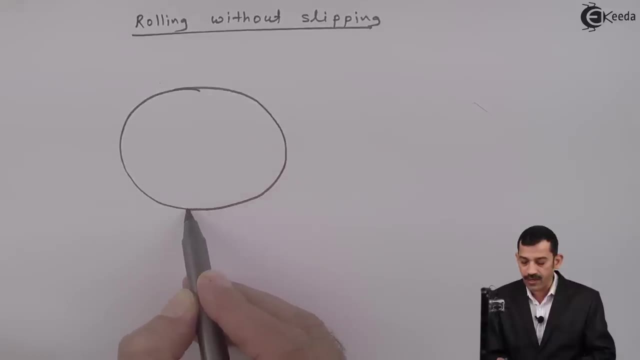 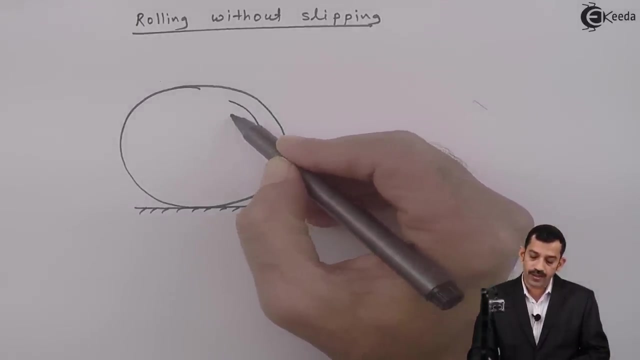 a circular body. you may assume this one as a circular ring, may be spear, may be cylinder, may be wheel, of any vehicle which one rolls without slipping. say this one is a ground here, will roll, say in some direction, say this is the direction of omega. now, which location represents here center of rotation? you know, center of rotation is. 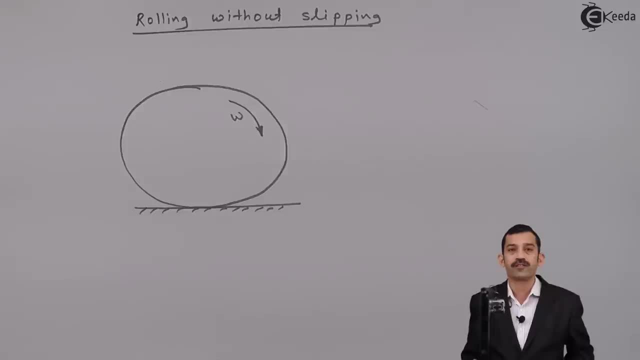 such a point whose linear velocity is zero, in this case center of wheel. if will represent here center of wheel doesn't represent center of rotation. what is the reason when any vehicle moves or wheel rolls without slipping, this center of wheel moves parallel. here, center of wheel doesn't represent center of rotation. 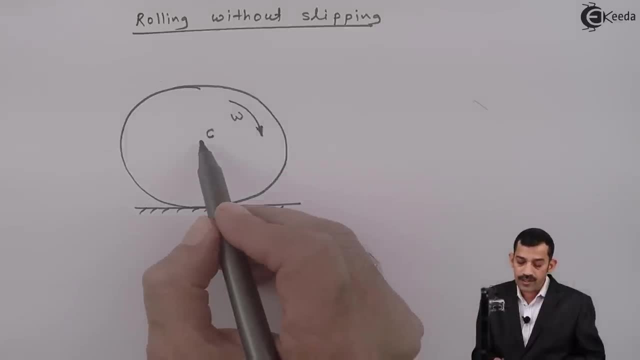 to the ground. that means, as omega is clockwise, this c or this linear velocity of point c, you will get in horizontal direction. any vehicle equals when it moves axle of vehicle, that one moves parallel to ground. that means as this one is a position of axle which is center. 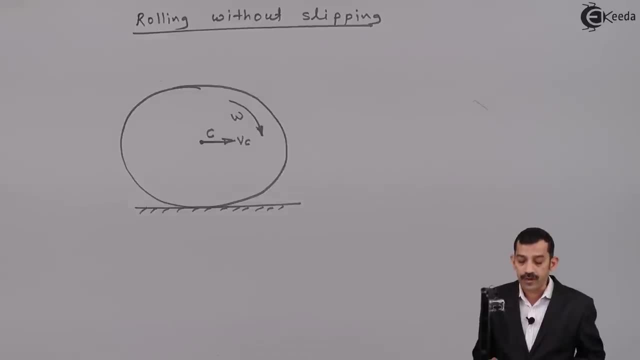 of wheel. it moves parallel to ground. now, meaning of rolling without slipping. that means at contact surfaces there is no slipping. linear velocity of ground is zero. that means the point on the wheel circumference of wheel which comes in contact with the ground. now, there is no slipping. that means the point which is in contact with the 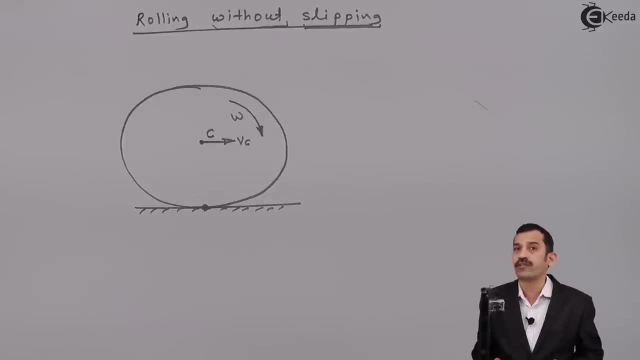 ground, its velocity must be zero, because linear velocity of ground is zero. otherwise if you'll assume some linear velocity of that point which comes in contact with the ground, if you'll assume some velocity, then there will be slipping. slipping is possible in some cases if you are. 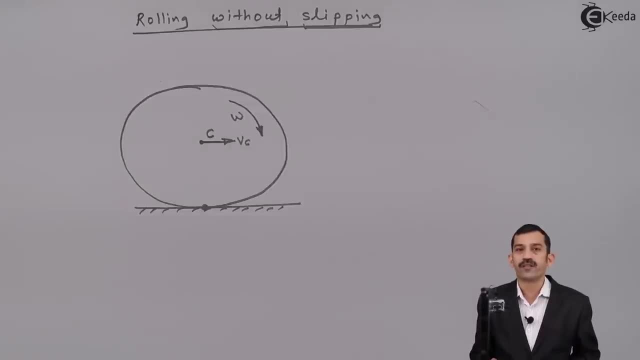 driving a vehicle and road is oily, slippery and suddenly, if you'll apply brakes, the vehicle skids. that motion is rolling with slipping. but for normal type of motion- rolling without slipping, as there is no slipping in contacts, at contact surfaces- linear velocity of ground zero. the point which comes in 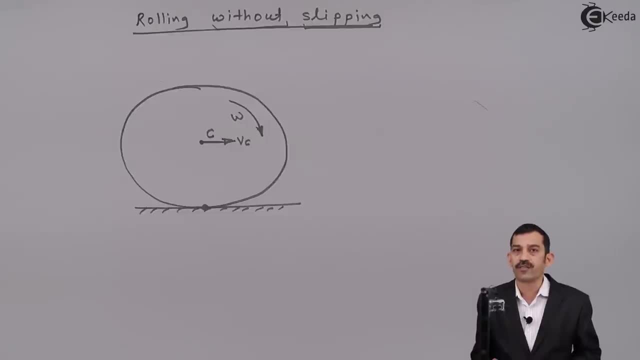 contact with the ground, its velocity at that instant becomes zero. therefore, this point of contact, what you are getting here, is icr. why name is given as icr? because, say, point a comes in contact with the ground. next one: this point again comes in contact with the ground, to this point moves away from the ground. that means 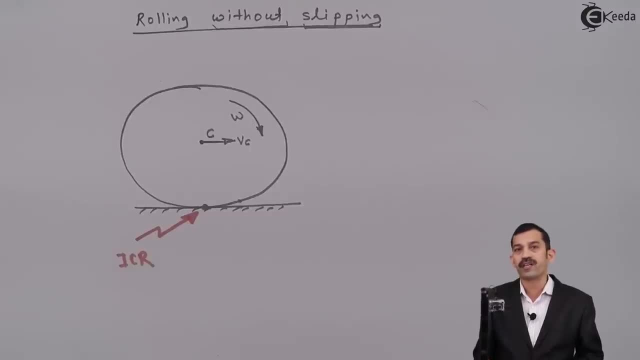 each and every point on the circumference of will becomes icr when it completes one revolution, but same point will not be icr at all the time instances as position of center of rotation changes, that point is always different. name of this point or center of rotation is what icr. now, if we'll join this point to this center and this will 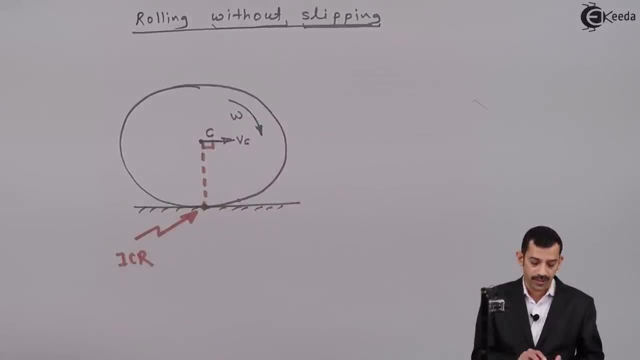 rolls in clockwise direction. velocity: linear velocity is perpendicular to radius of rotation. now if you say a represent linear velocity of any other point. say this one is one point, point d. how will represent center of rotation? the center of rotation is fixed. say point i: linear velocity of point d, if you want to represent it, is always perpendicular to radius. 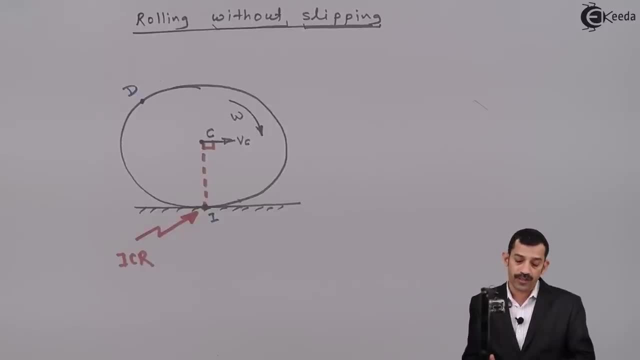 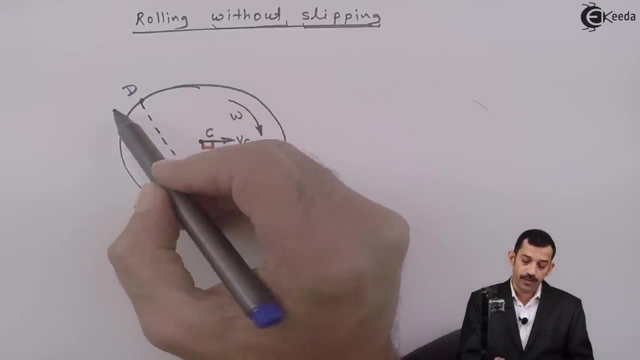 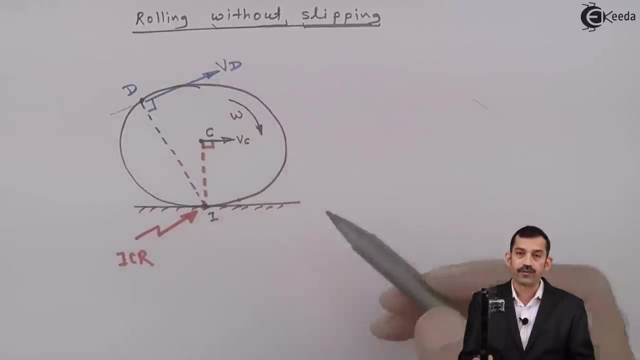 of rotation. that means i'll join point i to point d which represents what radius of rotation, as this one is, radius of rotation will draw perpendicular to radius of rotation. omega clockwise that means linear velocity of point d is what vd perpendicular to id. any other point is given. say this one is one more point. say point b. 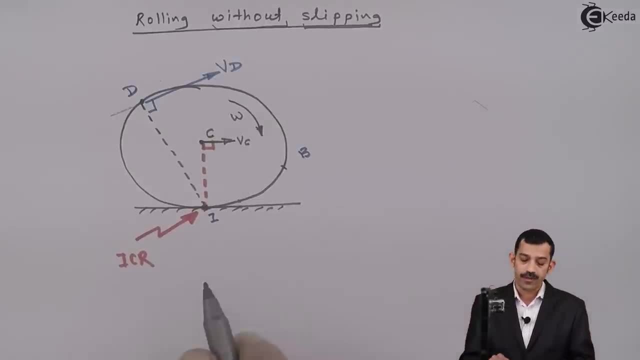 what is the linear velocity of point d? what is the direction of linear velocity of point b perpendicular to radius of rotation? which one is radius of rotation? i will join to point b, always concentrate. important point is center of rotation. if you want to find out linear velocity of any point on rigid body, that 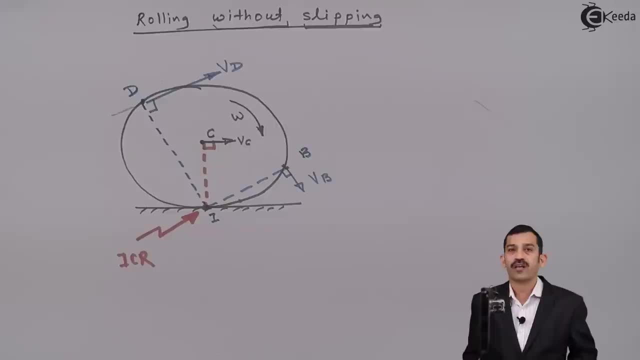 point will join to center of rotation and once will drop perpendicular to it we'll get linear velocity of any point anywhere. if you want to represent linear velocity of any point on the rigid body body, always join that point to center of rotation. will draw perpendicular to radius of rotation. 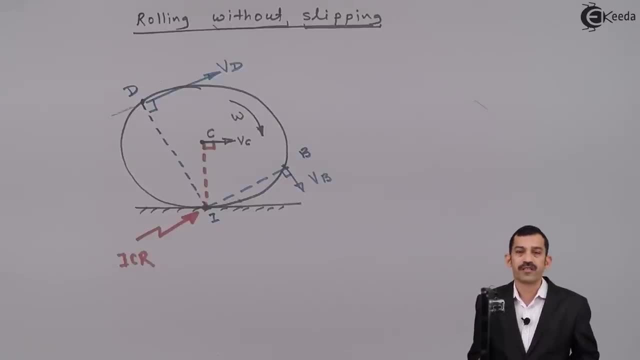 concentrate on direction of omega and in the same sense of omega will represent linear velocity of that point. Thank you.